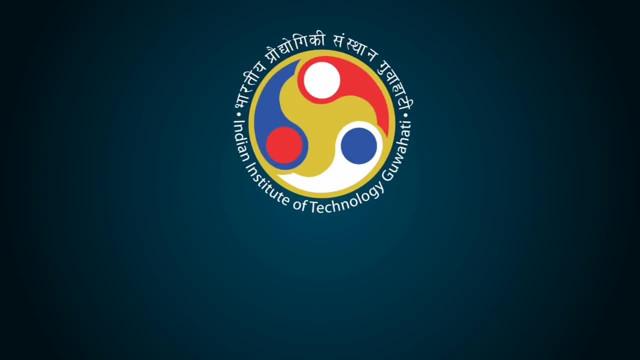 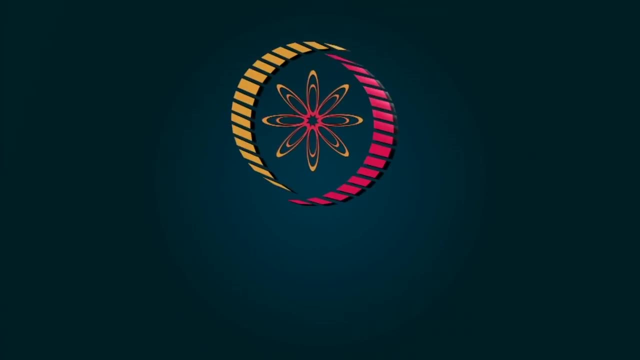 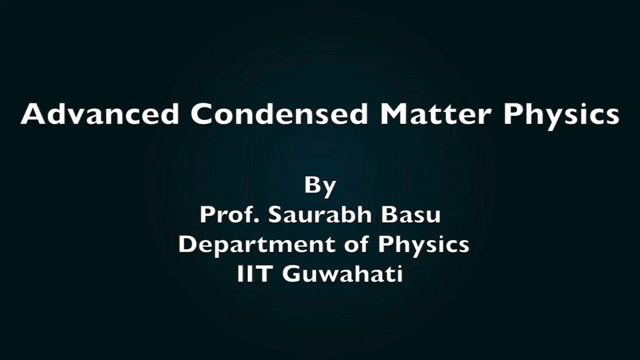 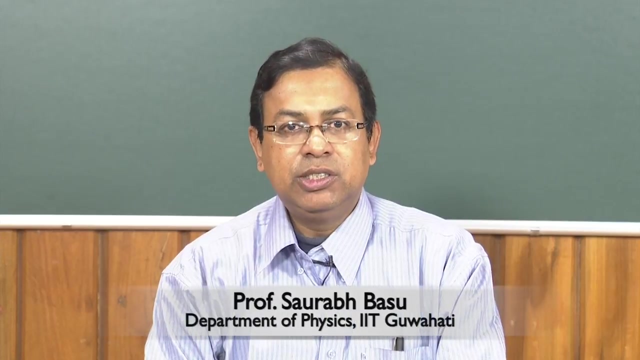 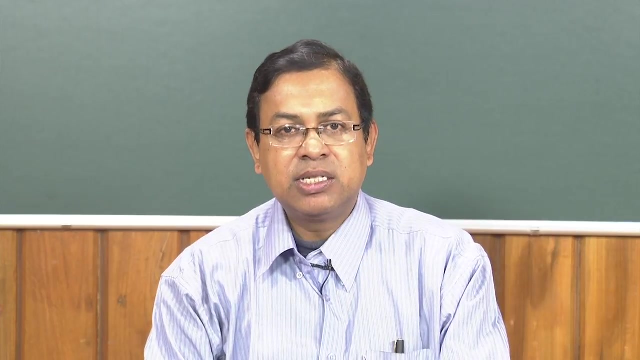 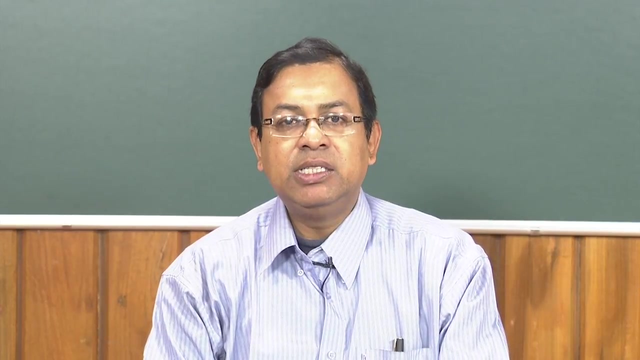 So in this set of special lectures we shall do quantum Hall effect to begin with, and then we will see that how it gets connected to more exotic phenomena. So we are familiar with Hall effect. Hall effect is an effect which was discovered in. 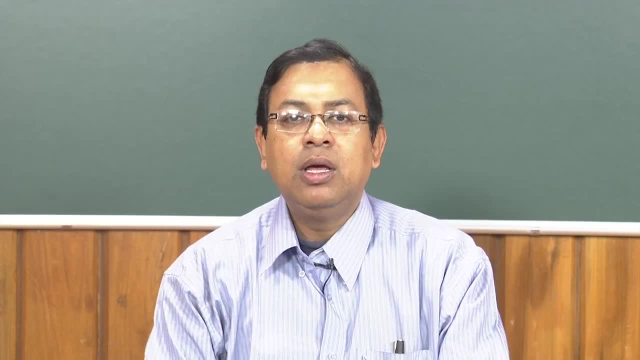 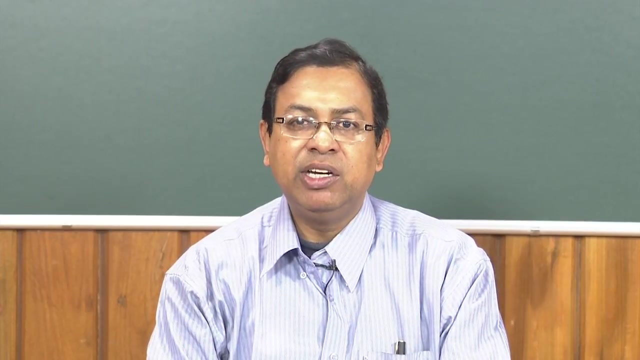 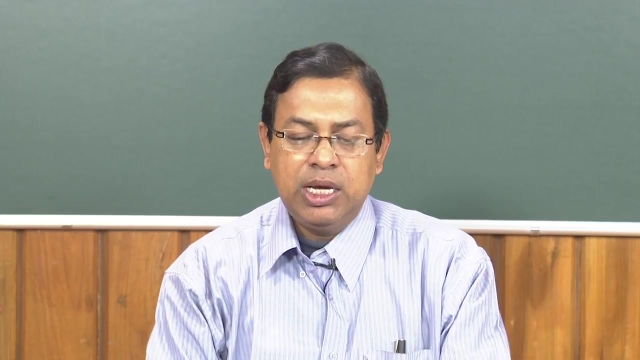 1879 by Edwin Hall, in which the current is made to flow in a thin laminar sample. So, for example, in, say, the x direction and there is a voltage that is generated in the y direction because of the migration of the charge carriers, abided by the Lorentz force equations and 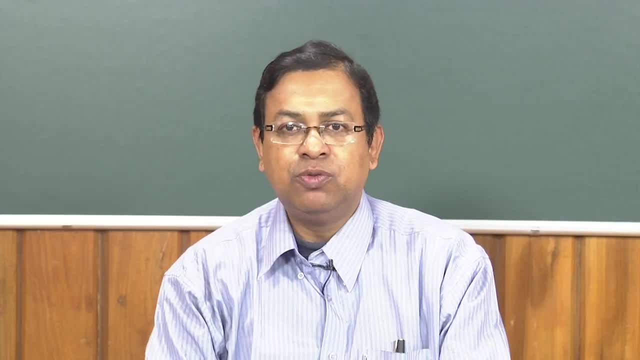 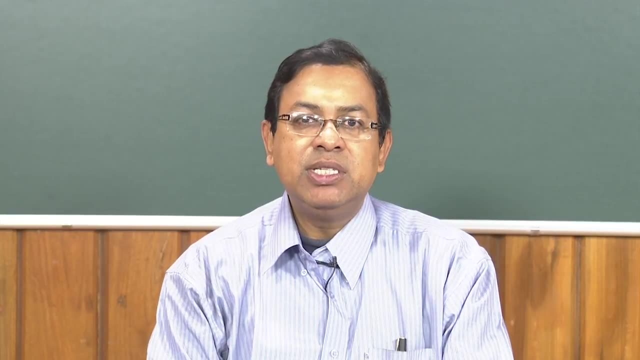 at equilibrium, one measures transverse voltage, which is known as the Hall voltage. So this is the quantum version of that and in which we will see that the resistivity versus the magnetic field plot which we have seen even in the classical Hall effect, Here there are. 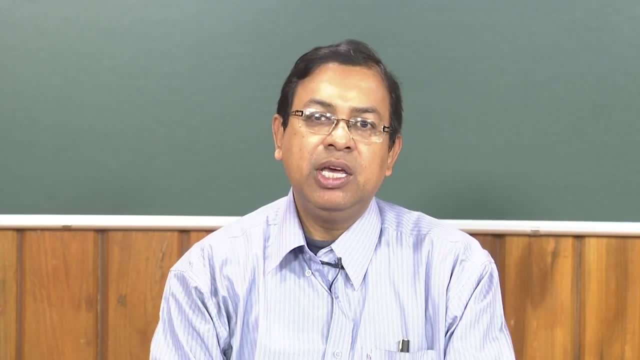 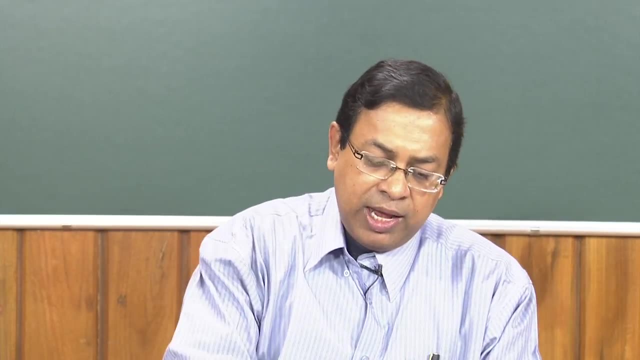 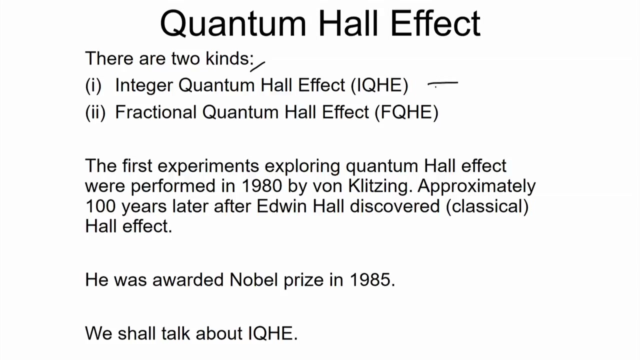 some strange features in this data and we will discuss that, how it comes about. So there are, in principle, two kinds of Hall effects, which are integer quantum Hall effect, which is what we are going to do mostly, and there are also fractional quantum Hall effect. 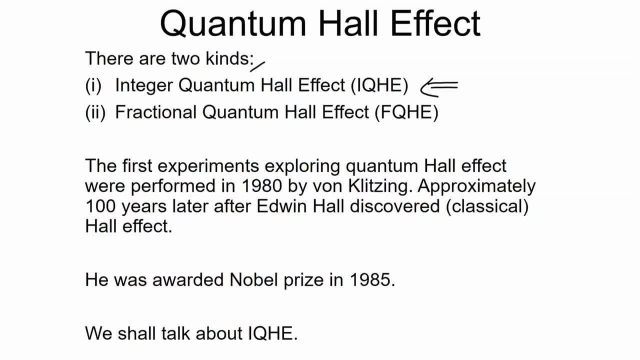 I will just mention what they are, But we will not get into the discussion because they are more difficult and they need interactions to be taken into account. So the first experiments exploring quantum Hall effect were performed by Von Klitzing in 1980 and then approximately, which is 100 years later, after Edwin Hall discovered. 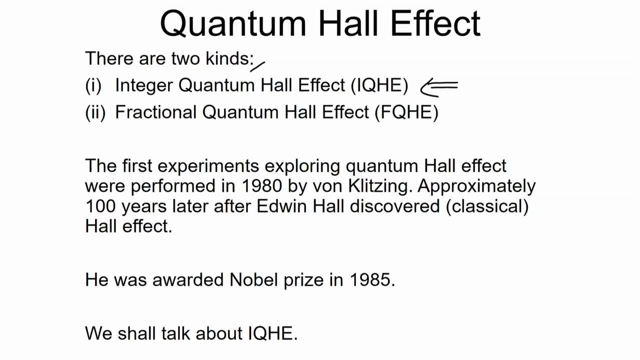 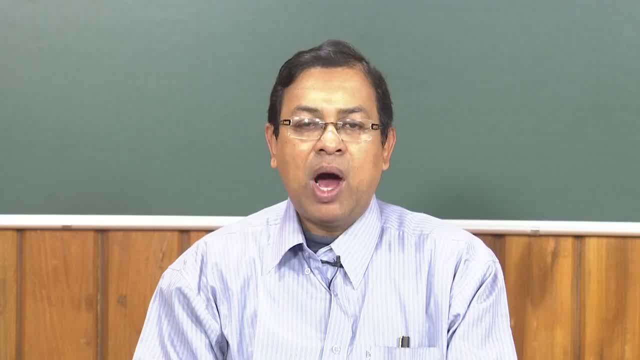 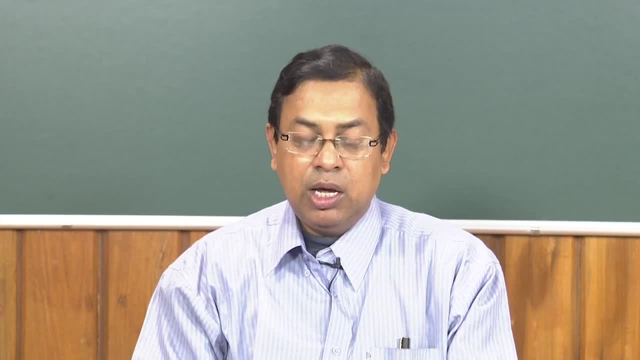 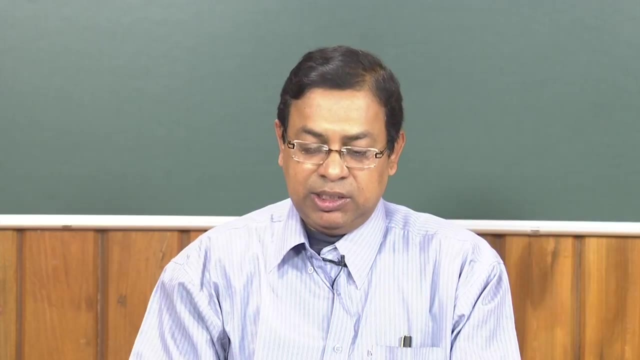 the classical Hall effect, as we have just mentioned, And Klitzing was awarded noble prize in 1985 for this discovery. So you will see that why this experimental discovery is so important so as to warrant a noble prize. So we shall talk about only IQHE, as I just mentioned. 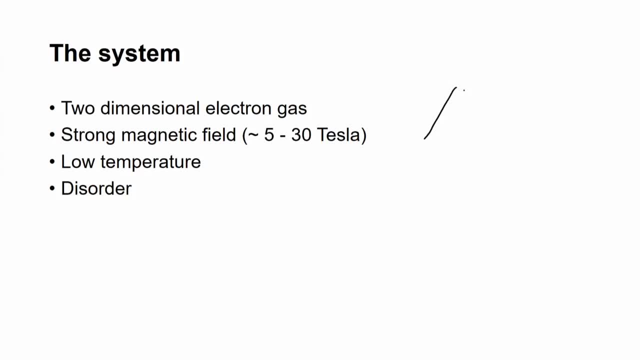 So what is the system? The system is a thin two-dimensional material, or quasi two-dimensional material, Video lecture on Quasi-Two-Dimensional Material and All-Methods of Electrical Exploration. electrons are restricted to move in two dimension and the extent in the third dimension is fairly 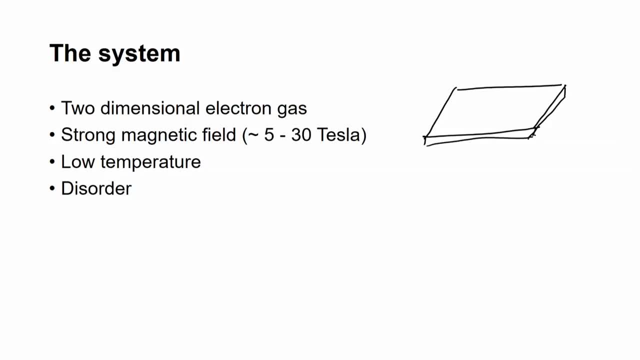 limited, So the motion is confined in the, in the plane. let us call it as x and this as y direction. So this is a two dimensional electron gas and it is written as 2, D, E, G in short, and there is a strong magnetic field that is been applied, which is perpendicular. 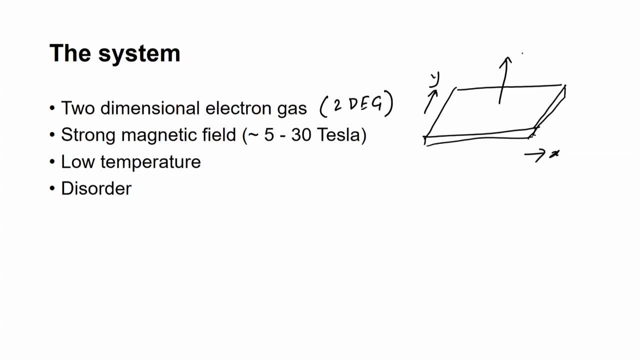 to it, So it is coming out of the plane. and this is the magnetic field- is of the order of 5 to 30 tesla. The experiments are conducted at very low temperature So that the quantum effects become important. Disorder is an integral part of this, of this effect or this experimental 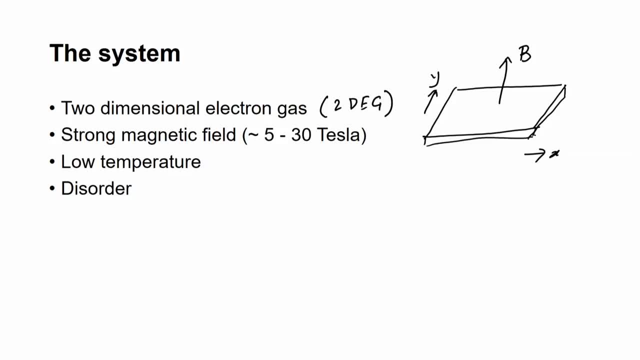 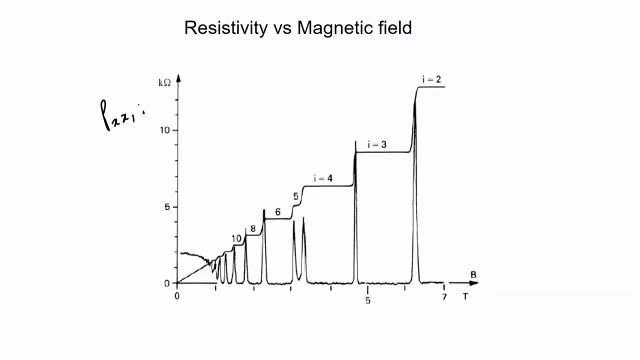 discovery and it plays an important role in seeing the phenomena better And in fact, in the absence of disorder, it can be shown that it reduces to classical Hall effect. So this is the plot of rho x x and rho x y. So let me point out which. 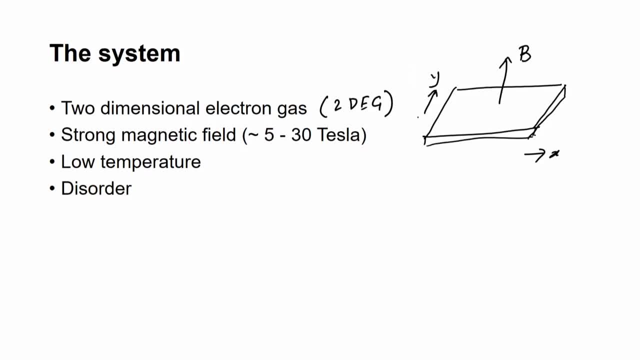 are the. So what is happening is that- So these, in this system, a current is made to flow in this direction- let us call it as J, x, and there is a voltage that is developed here, And that is why we can talk about either of either resistivity or resistance, And so 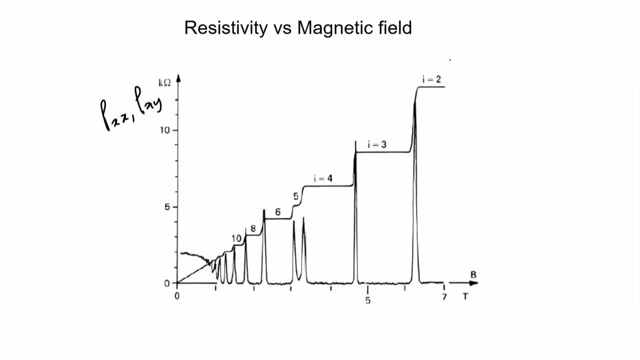 these are the plots for. So these step like plateaus are the plot for the Hall resistance, which will denote by rho: x, y, and these spikes that you see are for the longitudinal resistance or the magnitude resistance. So these are our plots. So these are our plots In the classical Hall effect, the Hall resistance or the Hall. 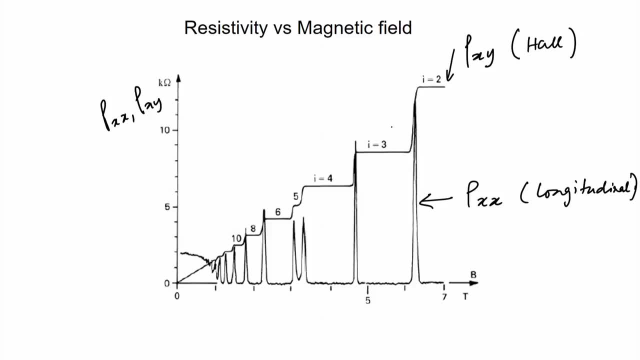 resistivity as a function of b was a straight line. Here it is far from being a straight line. there are plateaus at some integer values- we will discuss what that is- And at i equal to 2 and i equal to 3 and i equal to 4.. 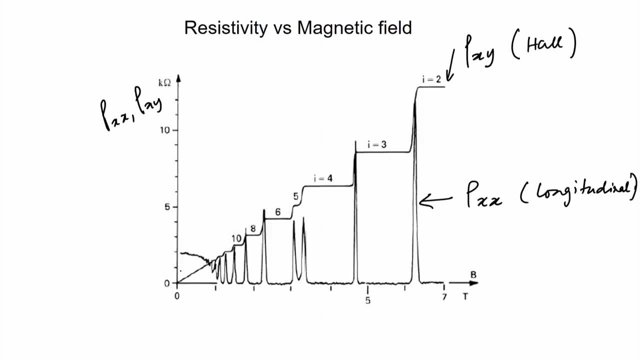 5. 8 and 10 and so on, And so these are in units of E square over, or rather H over E square. So the resistivity, the Hall resistivity for this plateau is 2 H over E square. this is. 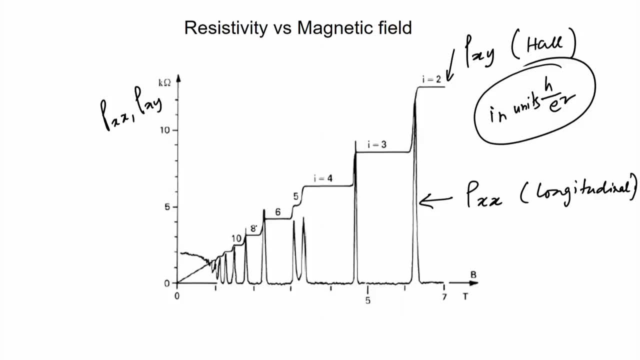 3 H over E square and 4 H over E square, and so on. Exactly that, and these integers are independent of the material, independent of the amount of disorder present, and is very, very universal. and so much so that these integers are correct up to 9th or 10 to the power minus. 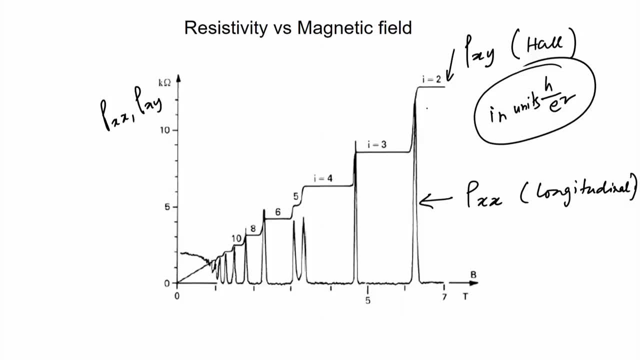 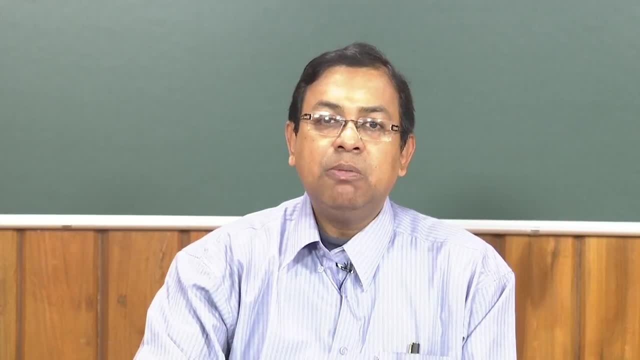 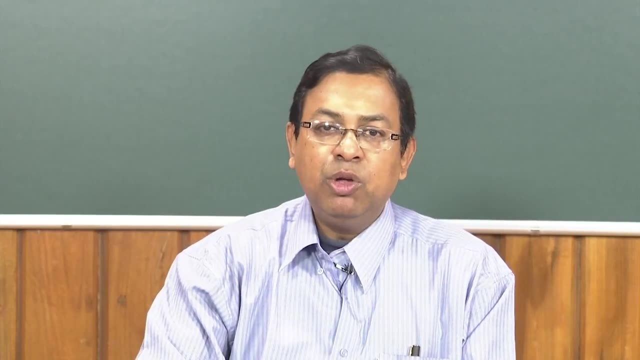 9 or 9 decimal places. So the effects or the experimental observations are that robust And absolutely independent of the material used, and hence this was really a discovery that has taken the scientific community by a storm, and at this lot of work since 1980. 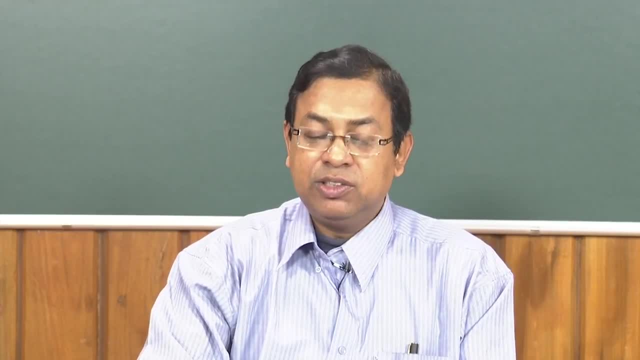 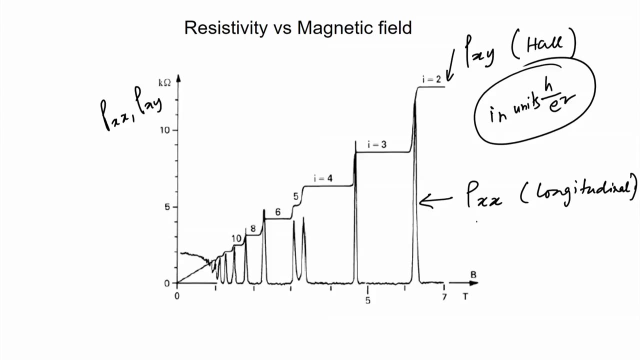 that have started and still going on in various fields. So this is another important thing about this resistivity that the longitudinal resistance is 0 most of the time But it shows a peak as the Hall resistivity makes a transition from one plateau to another. 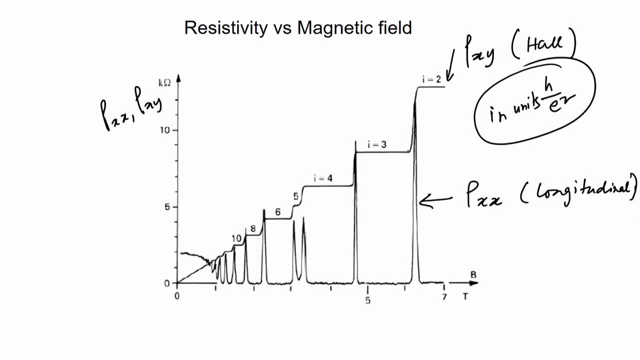 So it is only when it makes a transition from one plateau to another, it shows a peak. and you see, the peaks are all there, accompanied by the jump from one plateau to another. So you see the rho x, x, which is the longitudinal resistivity. 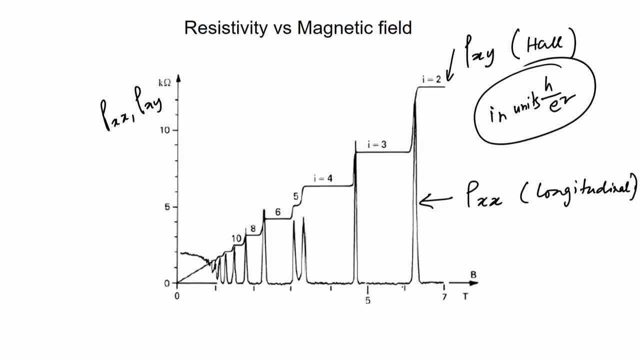 So there areWe see that another part of the resistance. if it is Rif Holder present, it is 0, which means that resistivity is 0. So Means it is a perfect metal or perfect conductor. and suddenly the thing: the resistivity shoots. 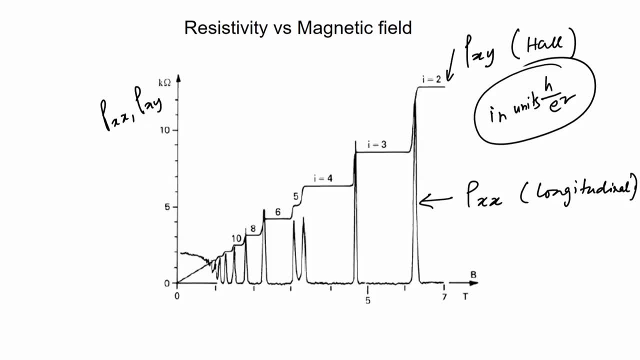 up giving rise that there is a lot of resistance there. So the will system over nat b. In fact there is not resistivity except for the ρ, which the R, and it gets larger as it erodes through a 30 degree angle during the heat transmission. So in that case the resistance. 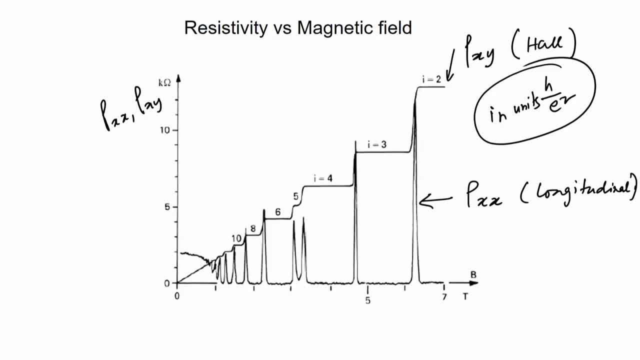 of the chemical resistance apartment goes more higheraltung, energy efficient S meilleur frequency of whatever it might be, and that is called finer frequency. that what we are thus of metal resistance That Since 때, even in Had down through Rs Jacques, is really 0.. 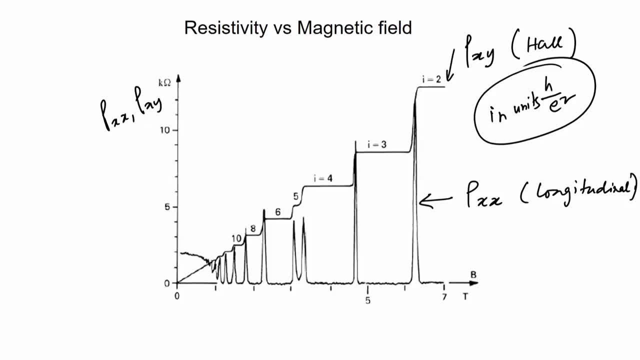 to insulator, to metal and so on. So these are some of the interesting features of the quantum Hall effect, which are which are very important and for us to understand that, what is going on. So, just to summarize that we have said this. 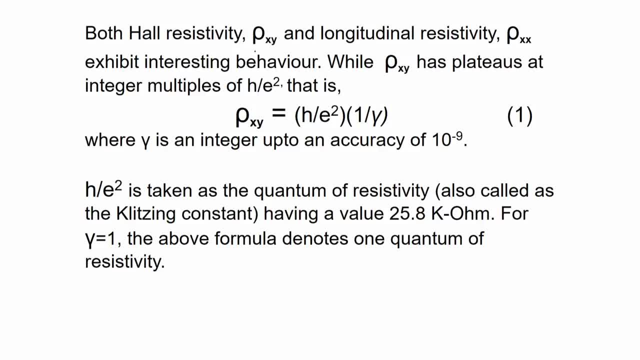 the Hall resistivity and the longitudinal resistivity. the Hall resistivity is given by rho xy and the longitudinal resistivity by rho xx exhibit very interesting behaviour, as we have just seen, while rho xy has plateaus at integer multiples of h by e square, that is, rho xy equal to h by e square and 1 over gamma, where gamma is an integer. up to an accuracy. 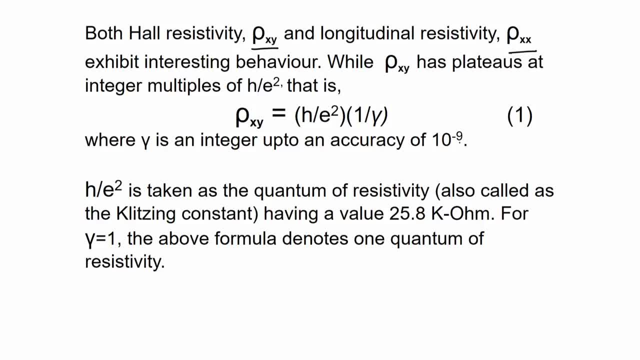 10 to the power minus 9.. And because of this robustness of these plateaus- and remember that we have said that disorder is an integral part of the system and since disorder does not do anything, So, which means the fact that translational invariant is broken does not have any effect, 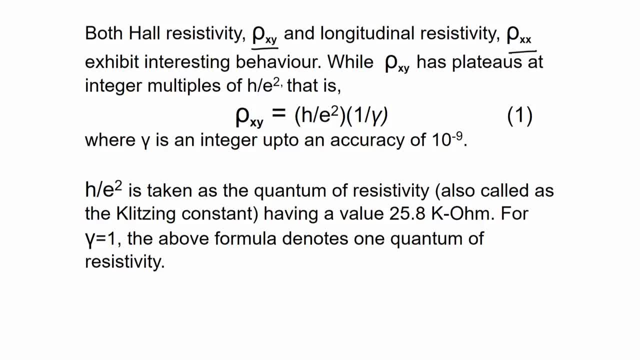 on this, So there must be some other mechanism that is, protecting the flatness of the plateaus. h over e square is thus taken as a quantum of resistivity, and it is also called as a Klitzing constant by the name of the discoverer. It has a value approximately 25.8 kilo ohm. 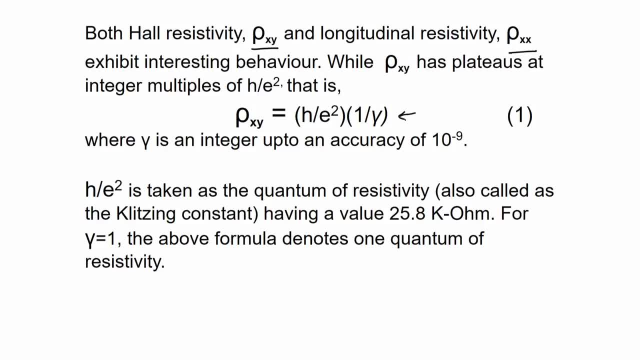 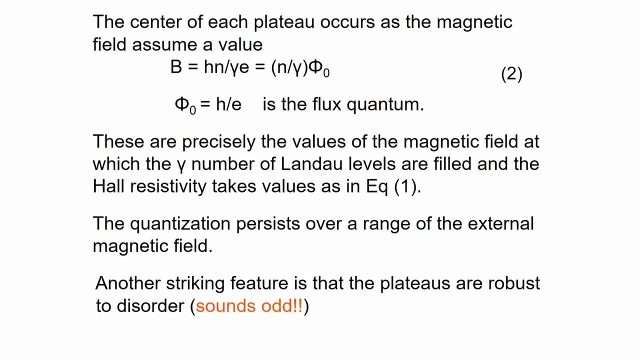 and you can see that for gamma equal to 1 here this denotes exactly one quantum of resistivity. So it becomes 1 over 1, which is just simply h over e square. There are more features which we unfold one by one. the centre of each plateau occurs at: 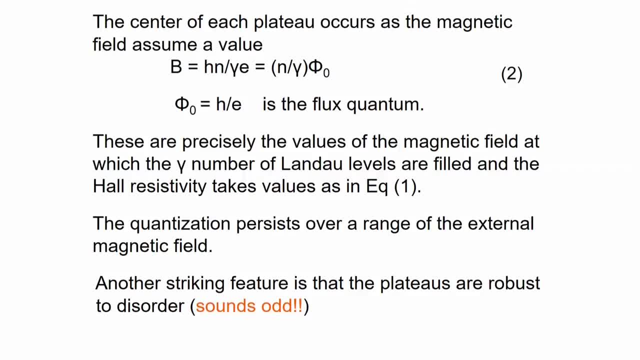 the magnetic, as the magnetic field assumes a value which is H- N over gamma, e Where gamma, where H over gamma, rather n over its n over gamma, and H by E, where H by E is called as a flux quantum. So as it takes a fractional multiple of this phi 0, or rather this some, 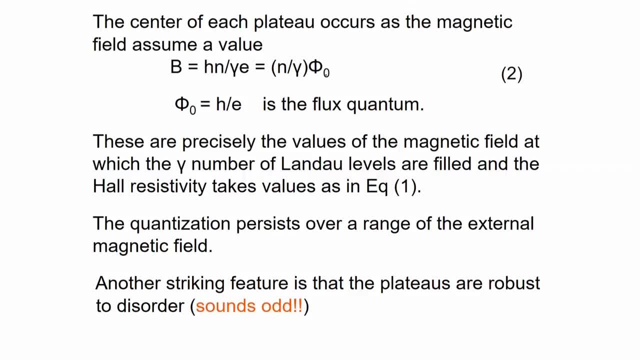 coefficient multiplied by phi 0, then that is where the plateau occurs. So it could happen that the value of the magnetic field n. So n is the density of the material, n is the electronic density. So what it is saying is that the value of the magnetic field 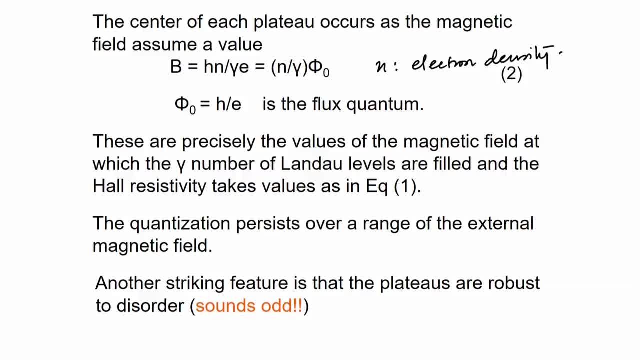 and the electron density Have to conspire to give rise to a plateau. So this is the flux quantum phi 0, which is equal to H over E. So these are precise the values of magnetic field at which the gamma number of Landau levels are filled. At this moment it is an unknown word, but we will. 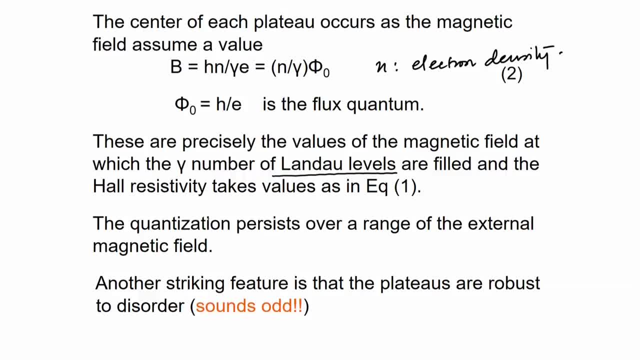 see what Landau levels mean, and the Hall resistivity takes a value, as we have given in equation 1, which is this: The quantization also persists over a range of the external magnet. So this is the magnetic field and another striking feature, which is we have already- 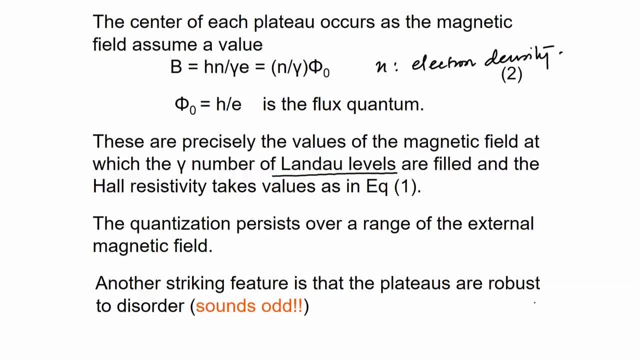 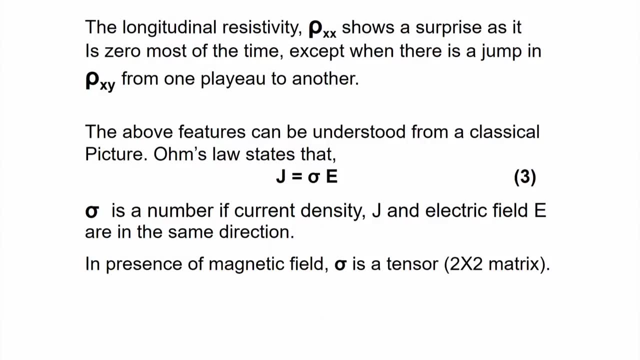 told is that they are robust to disorder, and it may sound odd in the context of condensed matter physics, because a large number of phenomena gets adversely affected by presence of disorder. while this is not So, the longitudinal resistivity, which is rho x, x, it shows a surprise, as it 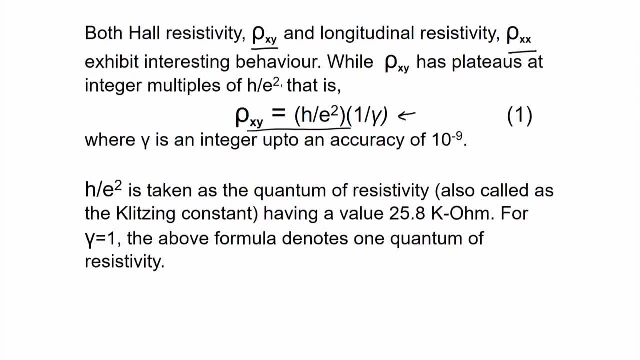 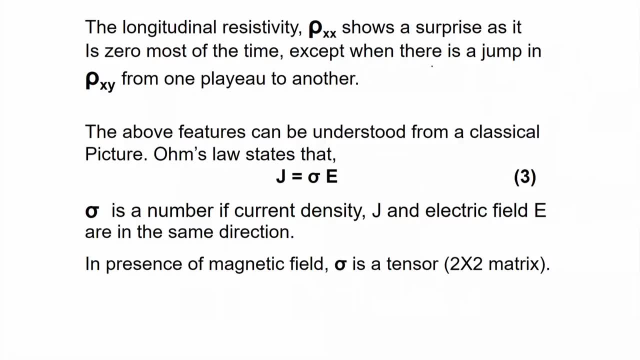 is 0 most of the time, as we have told. So it is 0.. 0.. Because we have 0 here, 0 here, 0 here and so on, except when there is a jump in rho, x, y from one a plateau to another. 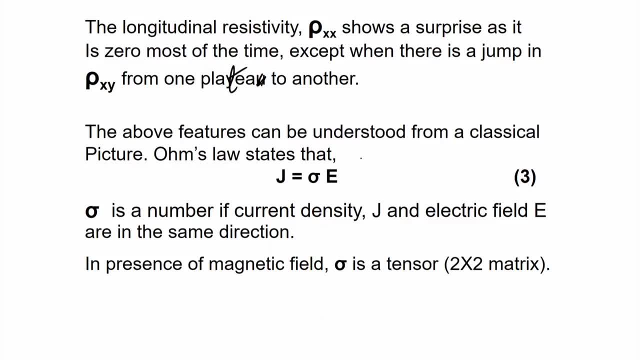 So the above features can be understood from a classical picture. So let us see what the classical picture unfolds in this particular case. It has got nothing to do with quantum mechanics, but these will help us in understanding states that J equal to sigma E. this is another way of writing. V equal to I, R, as everyone. 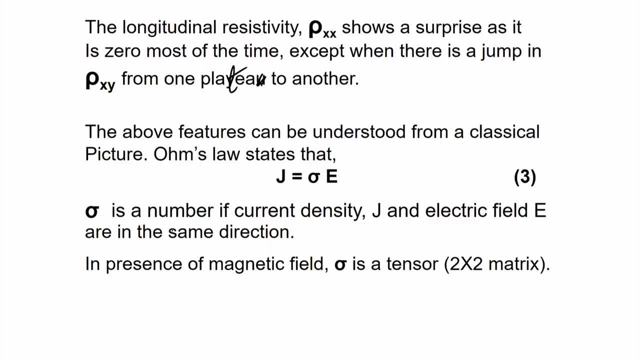 knows, sigma is a conductivity, So sigma is conductivity, J is current density and E is the electric field. So sigma is a number if the current density J and the electric field E are pointing in the same direction. So J, x equal to sigma, E, x and. 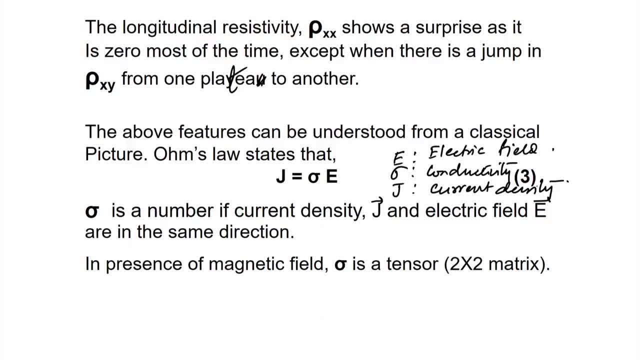 so on, and in which case sigma is a number, but in presence of a magnetic field sigma is a tensor. it is a 2 by 2 matrix having a form. So sigma is equal to Sigma x x, sigma x y minus sigma x y, sigma x- x. So it tells you that diagonal elements 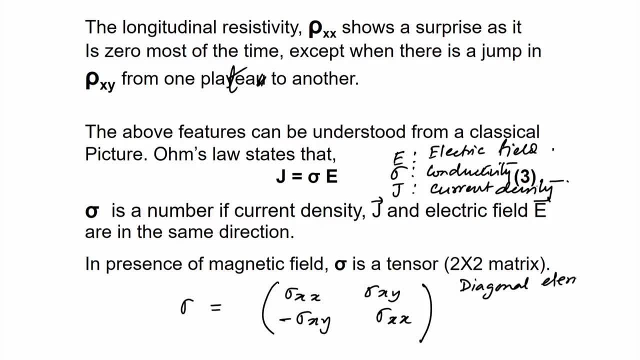 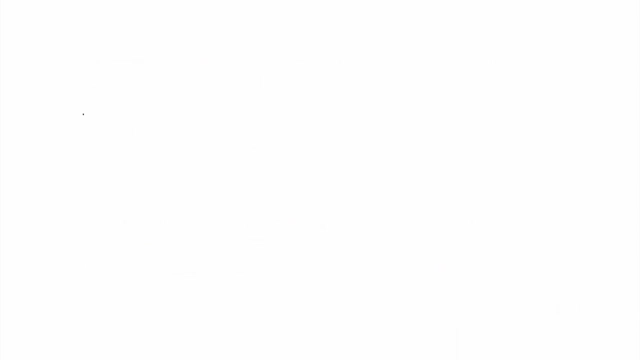 are same. off diagonal elements are anti symmetric. So these are the features of this matrix, and so if we write the conductivity tensor, we can also write the resistivity tensor. So the resistivity tensor is written as: So, which is equal to sigma inverse. this preserves the similar properties with an off diagonal. 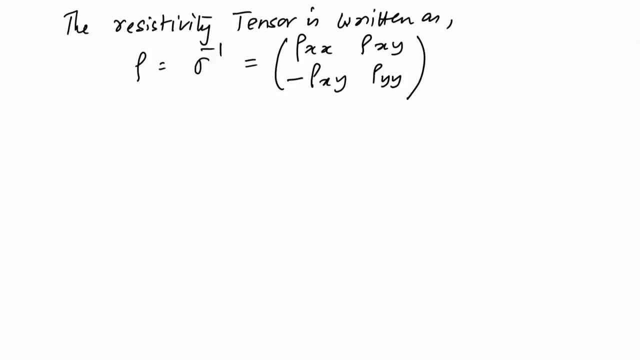 variance being anti symmetric. So the it is easy to see that the components have the relation that sigma xx, equal to rho xx, divided by rho xx square, plus rho xy square, and the off diagonal Elements have minus rho xy divided by rho xx square plus rho xy square. Now if rho 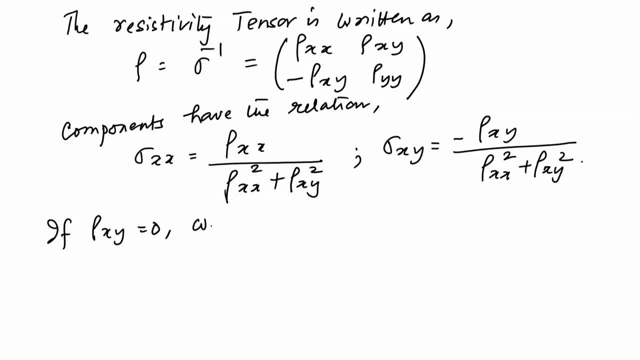 xy equal to 0. then we get sigma xx equal to 0, sigma xx equal to sorry, sigma xx is not equal to 0, but sigma xx is equal to 0. So this is 1 over rho xx. So this is familiar. and sigma xy is equal to 0. So this is 1- 2. 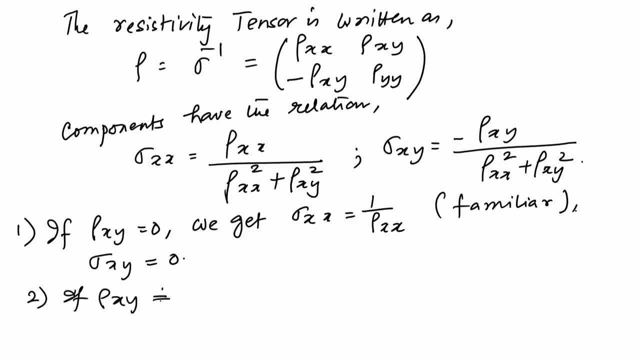 is that if rho xy is not equal to 0. Since sigma xx and sigma xy both exist, So this is clear to easy to see, that if rho xy is not equal to 0, then both of them will exist, and provided, of course, your rho xx. 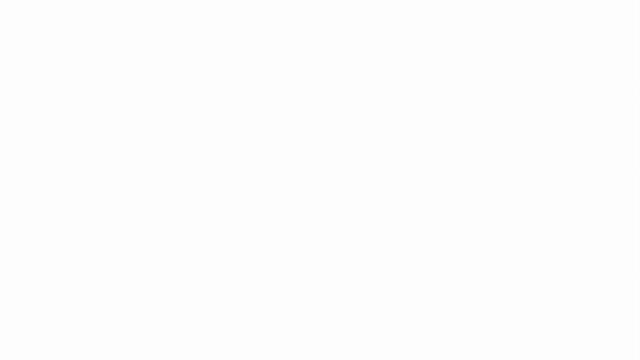 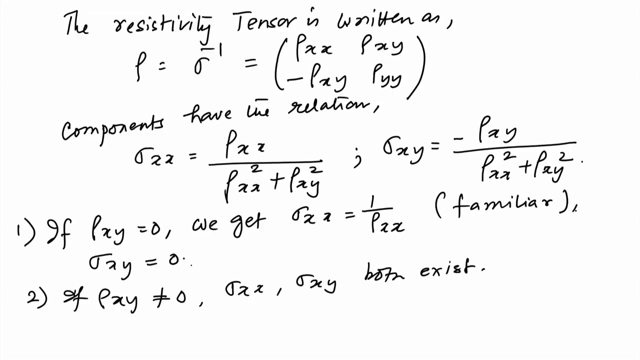 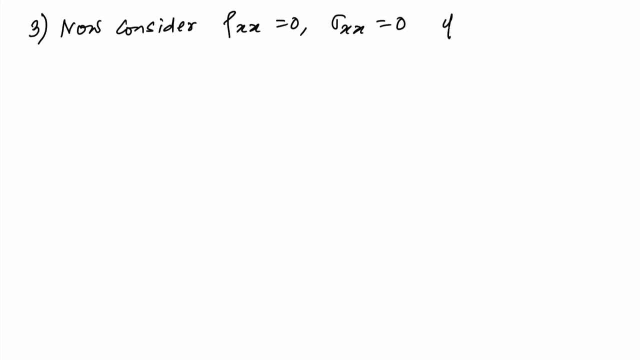 is also not equal to 0. xx is equal to 0. So sigma xx equal to 0. So that is clear from here. if rho xx is 0, then sigma xx is equal to 0, if, of course, rho xy is not equal to 0. So what do we want? 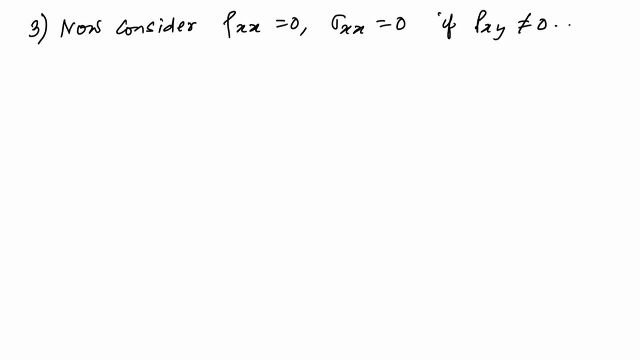 to call the system with rho xx equal to 0. So we have rho xx equal to 0, sigma xx equal to 0. on one hand, this tells that it is a perfect conductor and this says that it is a perfect insulator. 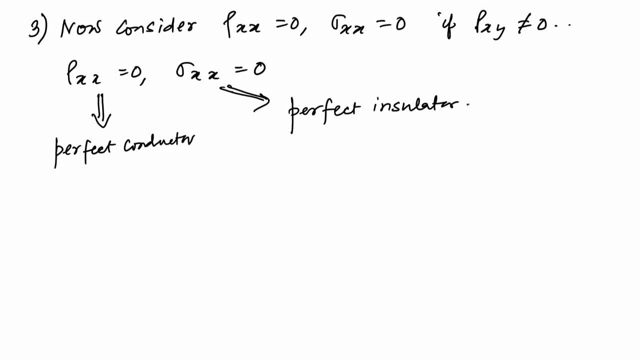 So one is implying the other, but one inference is that it is a perfect conductor. the other inference is that it is a perfect insulator. So the question is that: what is going on? and in order to understand this, let us just look at the Drude's model. 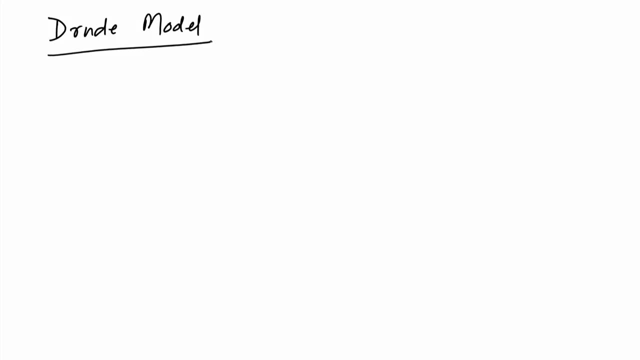 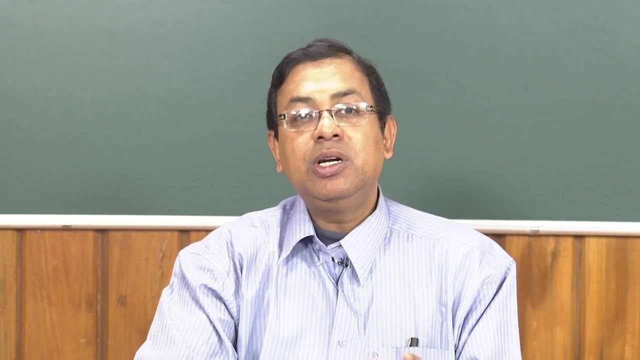 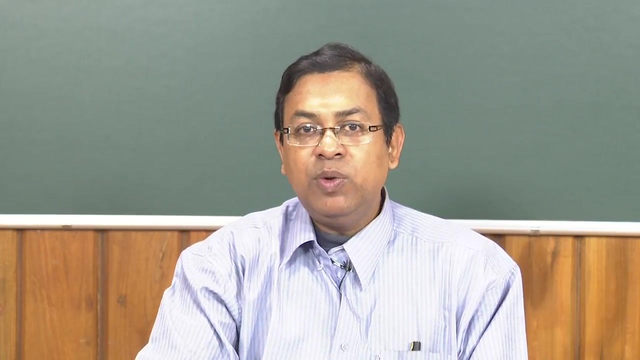 So in the Drude's model, this in the preliminary solid-state physics course, where, in the free electron theory, you have studied Drude model, which gives you the assumption that the electrons are non-interacting and they only interact when they collide with each other, which happens. 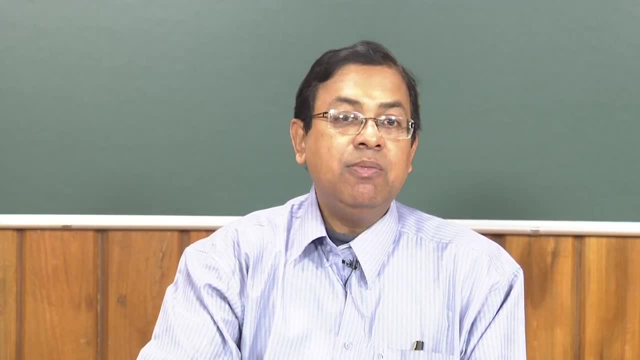 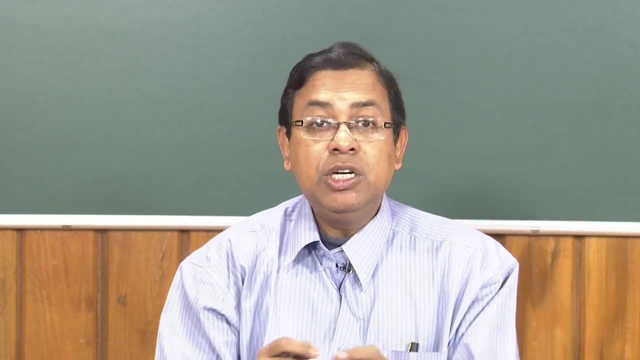 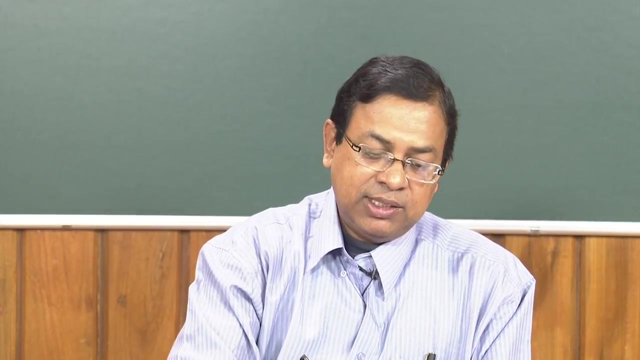 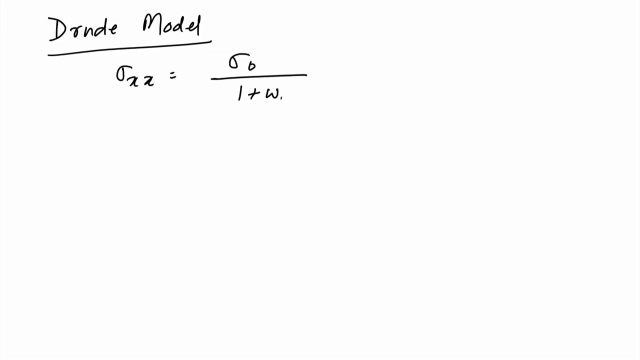 after every time motivation scale given by the relaxation time. So between these relax 2 scatterings, the electron propagates as free particle. So that is the assumption and the conductivity is given by 1 plus omega c square, tau square, where tau is the relaxation time, given by L, by V, f and omega c is some. 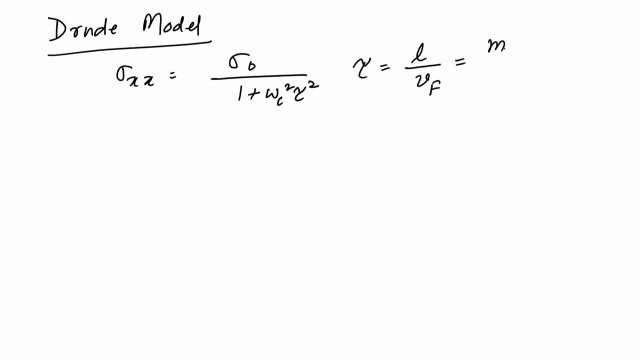 cyclotron frequency, where L is the mean free path and this is the velocity, And sigma 0 is taken as N e square tau over V, f, So M, with N as the density, M being the mass. So thus sigma xx equal to 0 imply that the 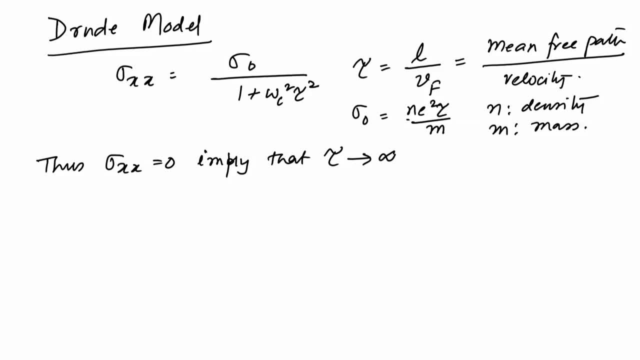 relaxation time becomes extremely large. So that tells that no scattering. So in this particular case, the current current is flowing perpendicular to the field, So that means it is very small and it has a form which is- we are talking about- two dimensional. 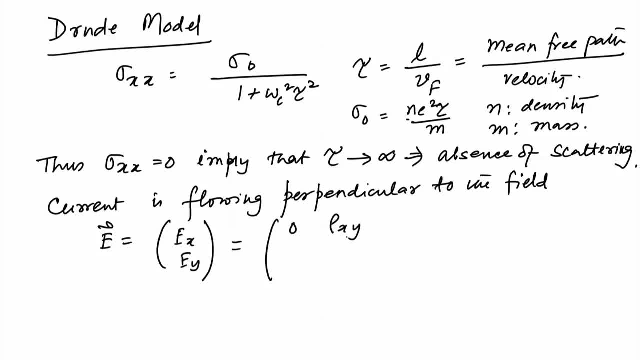 transport. So this is like 0 rho xy, because rho xs is equal to 0 minus rho xy, and 0 and jx jy, and this is equal to rho xy, jy and rho xy jy. So it is easy to see that that the E x is, so jy is in the direction of E x and jx in. 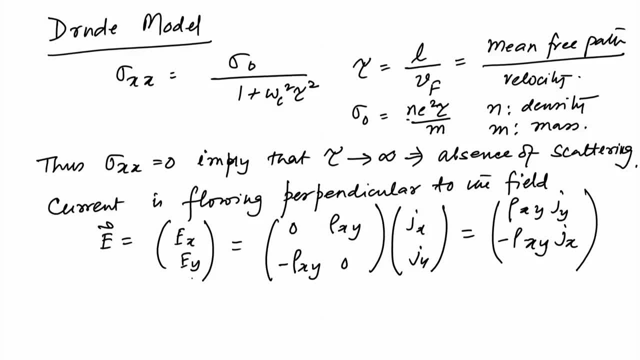 the direction of opposite to the direction of E, y, and that tells that E and j are perpendicular vectors. So if E and j, that is, the electric field and the current density- are perpendicular, then E dot j equal to 0.. So that is the electric field and the current density are perpendicular, then E dot j equal. 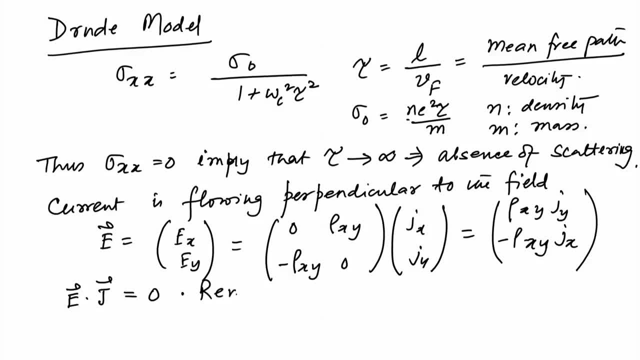 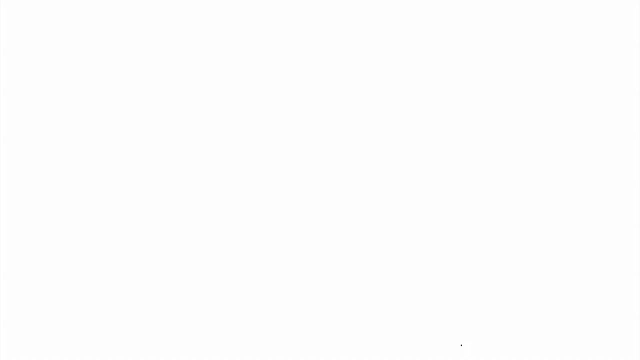 to 0, but remember that E dot j has the meaning of work done in accelerating the charges, And so the fact that E dot j equal to 0- it means that there is a steady current- implies that there is a steady current flowing in the sample. 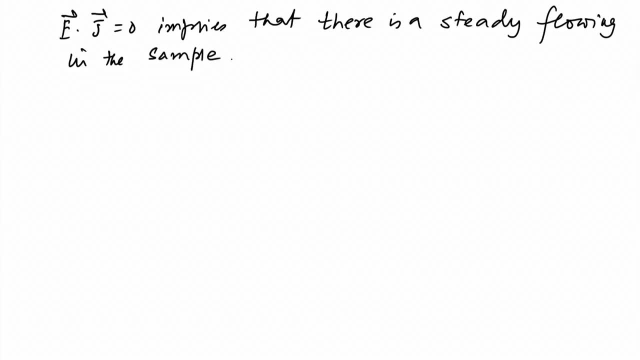 So that means that there is a steady current flowing in the sample which does not require any work to be done and hence no dissipation. So sigma x, x, equal to 0, and that is the E to 0, tells us that no current is flowing in the longitudinal direction. So this is like 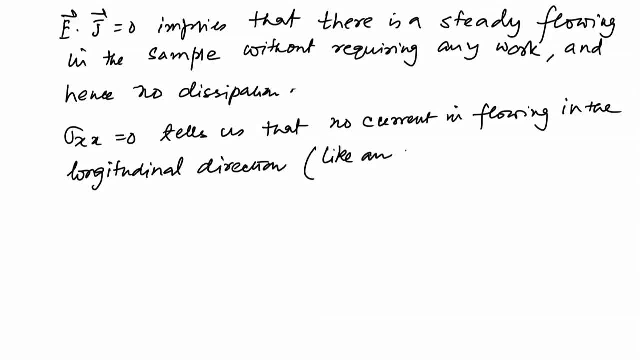 an insulator, while rho xx, equal to 0, tells that there is no dissipation of energy. So this is the like a perfect conductor. Let me add the word perfect here, also like a perfect conductor. So rho xx, equal to 0, equal to rho xx, is accompanied by that sigma xy, equal to minus. 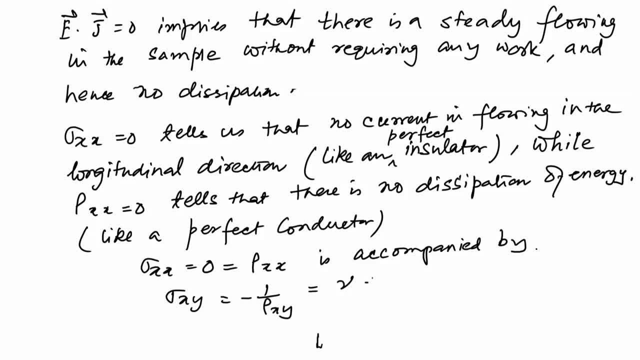 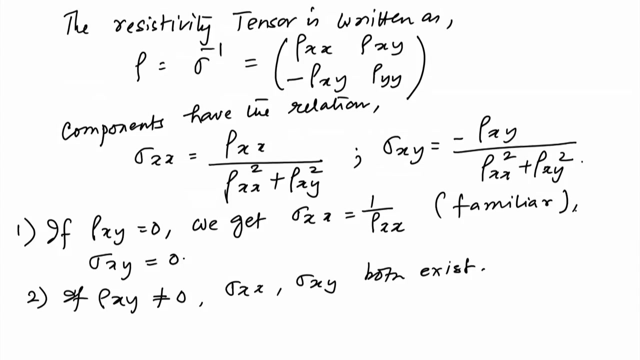 of rho xy, equal to nu, E square over h, and nu being an integer. So this quantization of nu being an integer to the accuracy of 10, to the power minus 9, is independent of the details of the system and hence the effect is universal. So this goes back to this plot. 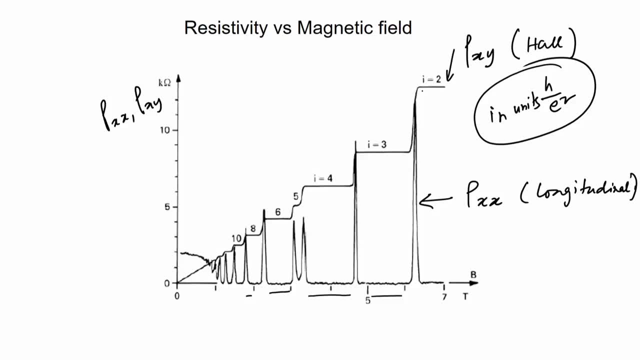 So this plot tells exactly that the rho xy will become a quantized number in units of h over E square, and it will make a transition from one plateau to another and during which the longitudinal or the magneto resistance, longitudinal resistivity of the magneto resistance. 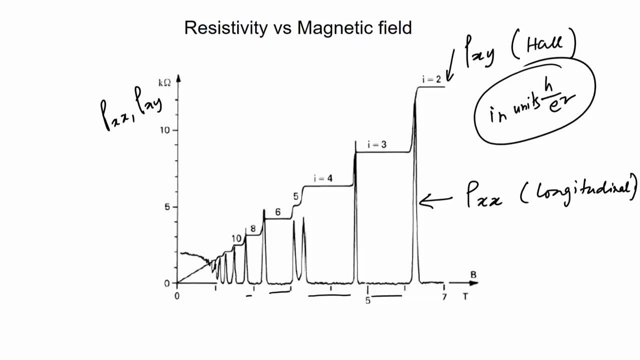 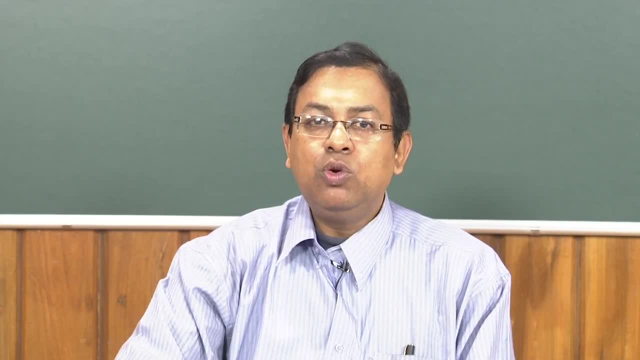 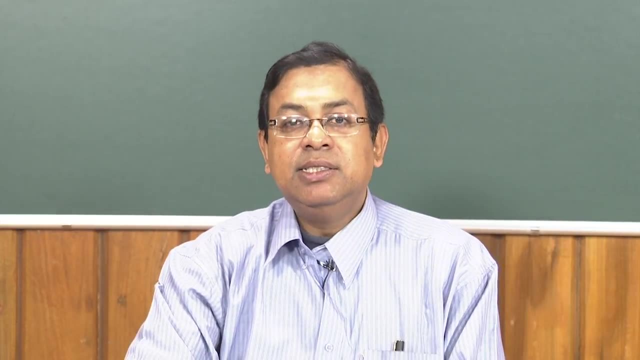 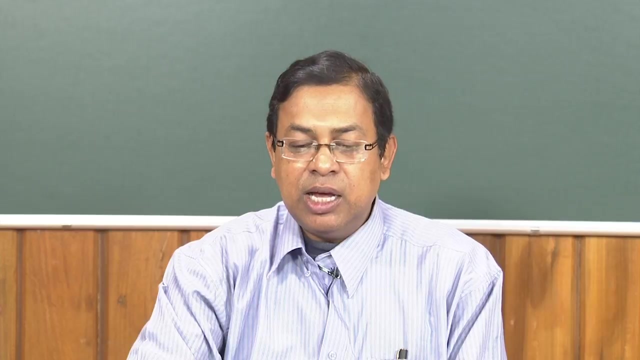 will show a sharp peak, and this, at least qualitatively, explains that these are universal features of a two dimensional electron gas, and persists even in presence of disorder. An important thing is that, since disorder is not protecting the plateaus, that is, it is get, or rather it. 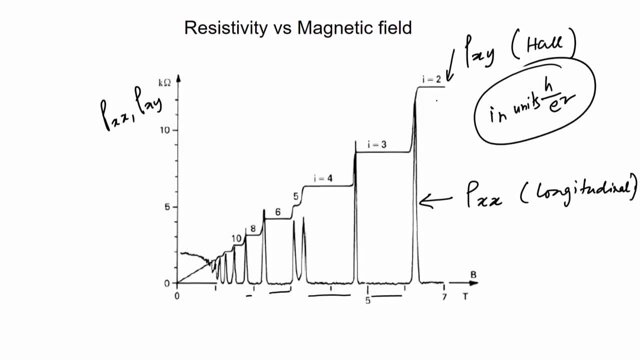 is contributing to the robustness of the plateaus, as we have seen, and magnetic field already has broken time reversal symmetry. So there has to be another quantity or another, you know sort of preserving factor that preserves. 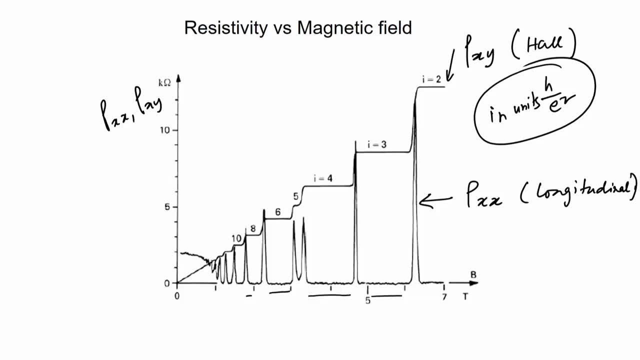 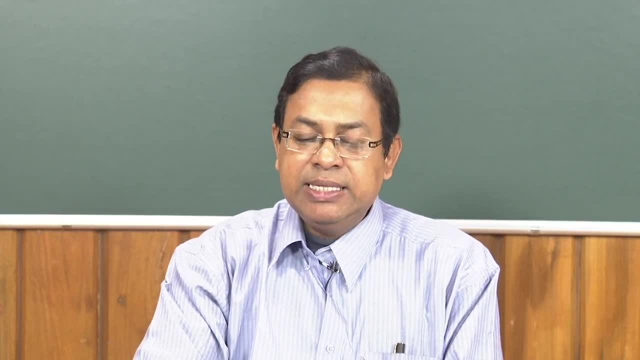 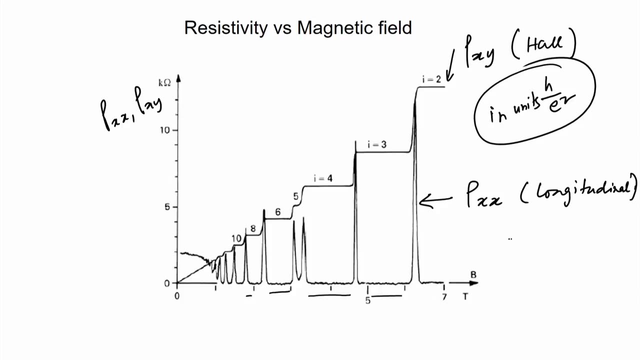 gives it a certain form of resistance, then it will absorb this plateau, and which is what has been attributed to the topological properties of the system that is protecting these plateaus. also, what happens is that in presences of the magnetic field, So the electrons go around in such circular orbits. 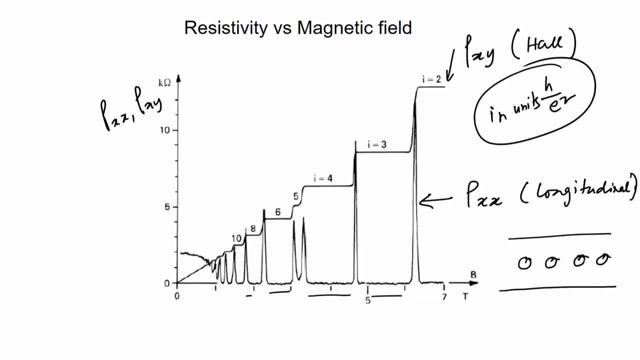 and the radius of this, or rather radii of this, orbits are proportional to the magnetic field. 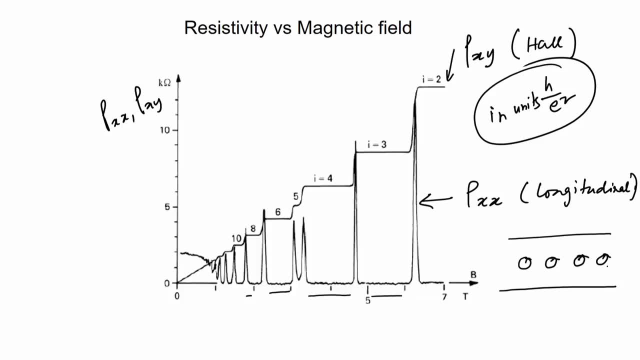 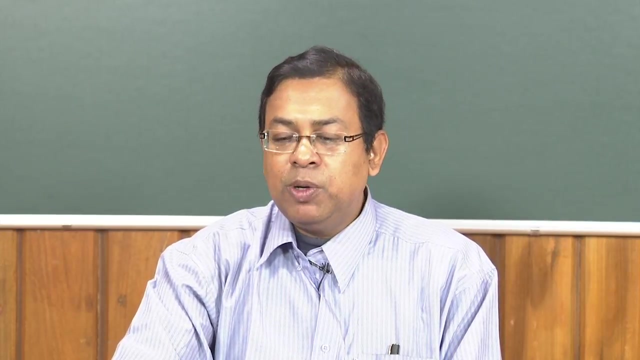 So this does not lead to any transport. but, however, the transport occurs along the edges, where the electrons actually skip, and these edge states are robust, no matter whatever a kind of perturbations you put. So these edge states will be robust and will carry. 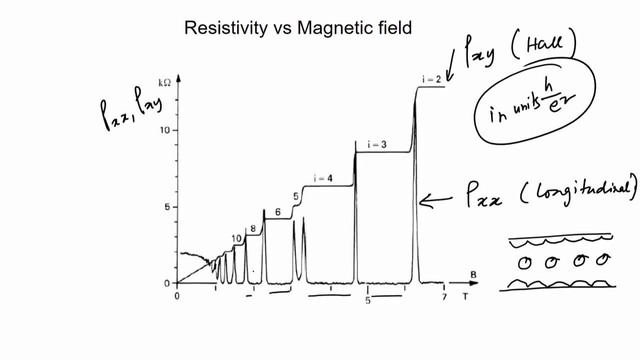 current and will give rise to this resistivity curves, while the bulk of the material that is interior of the two dimensional electron gas, the electrons, will not contribute to any transport of charges. Let us try to understand these features better and let us talk about simple language. 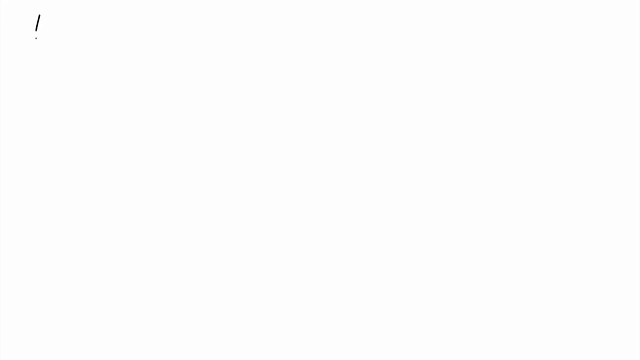 In simple language it is a non-interacting. So we want to talk about Landau levels. so electrons in a magnetic field. So these are non-interacting electrons in a magnetic field. So remember what happens in for a charged particle. 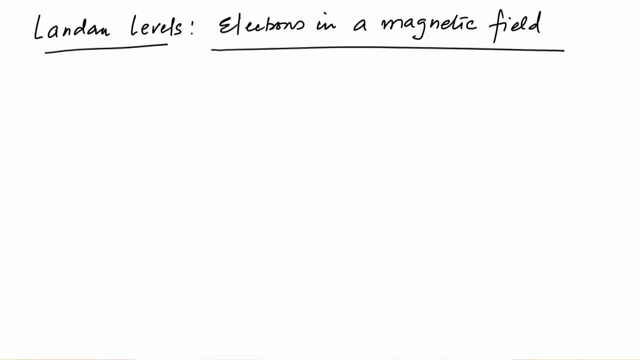 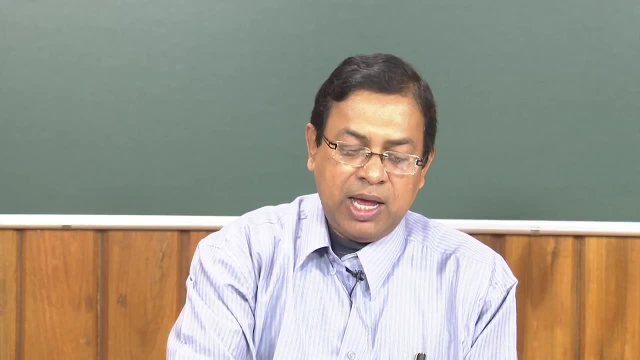 So remember what happens in for a charged particle. So you can see that with anерхitel janganicos of a weight, only then you have these費 going on. é particle to be put in a magnetic field. The canonical momentum P gets replaced by P minus. 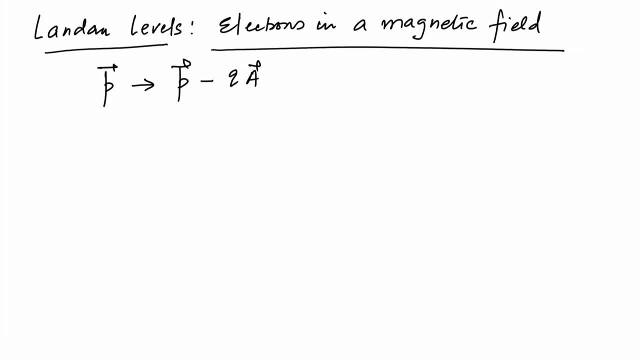 Q A over. well, this C will drop. those are old units. we can work in new units. and now Q is equal to minus E for electron, So we can write this as P plus E, A, where A is the vector potential and it has a relationship with the magnetic field given by curl, A equal to B. 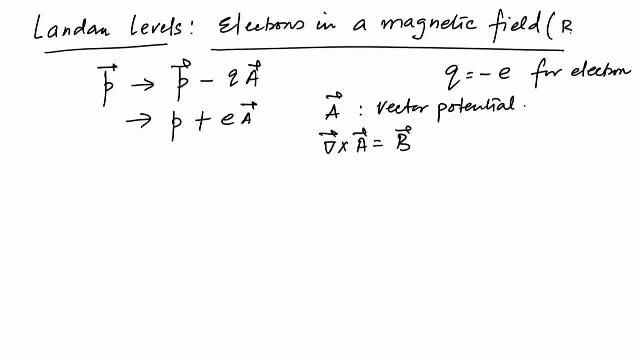 that is the magnetic field we are talking about. ok, So the Schrodinger equation that we have to solve is 1 over 2 m P plus E, A square psi equal to E psi. So that is the time independent Schrodinger equation. 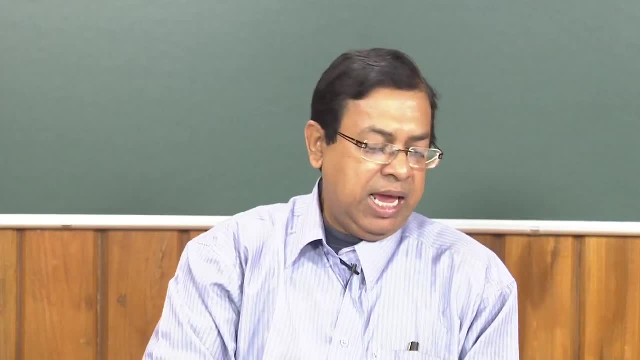 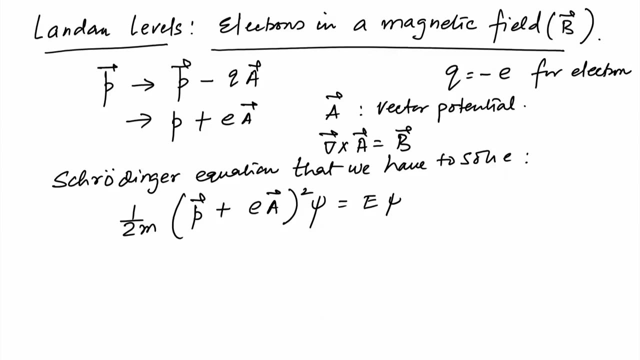 Where the P has been replaced by P plus E, A now Schrodinger equation is gauge invariant. So even if we change A to A minus, A minus gradient of a scalar function, we call it chi and arbitrary scalar function, which is the function of R only. Then psi simply picks. 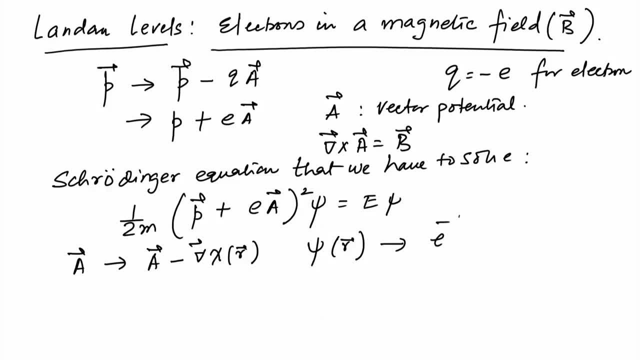 up a sign, Then it takes a motion of sign which is given by and because if psi picks up only a sign, only a sorry phase. not sign, it is a phase. this quantity, which is a physical quantity, remains invariant. So just to revise it once again, that we write down the Schrodinger equation: the A is a gauge. 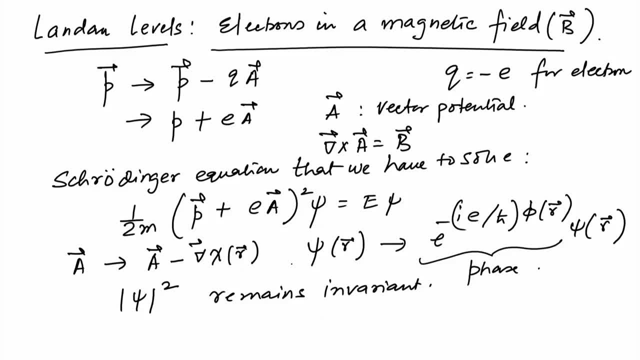 invariant and because of the gauge invariance, psi picks up a phase of this form. because psi only picks up a phase and not anything else, the psi mod square will not have this phase because it is psi mod square, is psi, star psi and you will have a simple you know. 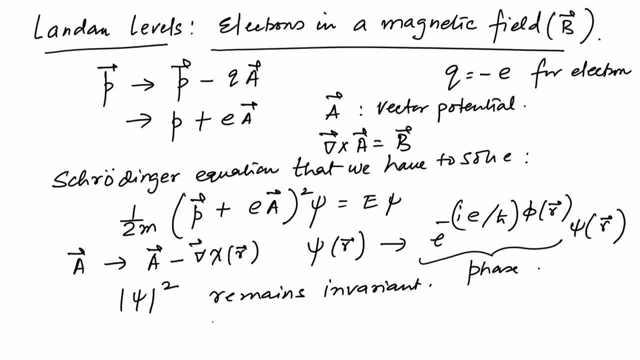 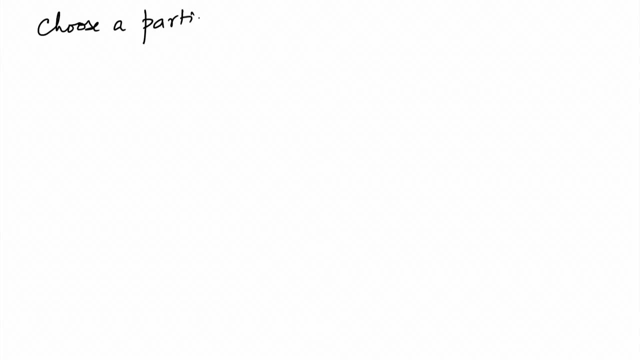 these will be same and hence we can do a gauge transformation on this and still get the same result. So now choose a particular gauge for calculation, and that gauge is, let us call it A x equal to minus B y. So the component x, component of A, is equal to. 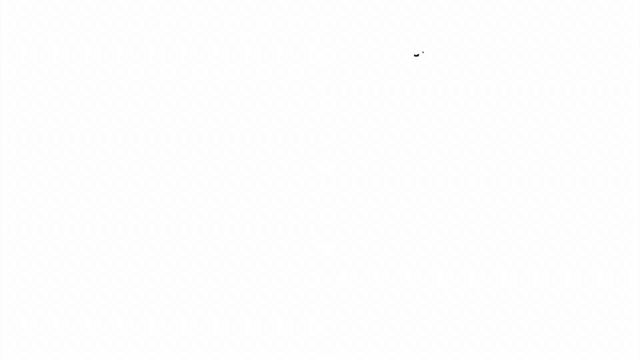 minus B, y, while the y component and z component to be equal to 0. This is called as the Landau gauge. that is the definition. This is fine, because curl A is B and so B is in the z direction, as is the requirement of the Hall effect. So we have taken, in principle, we have taken 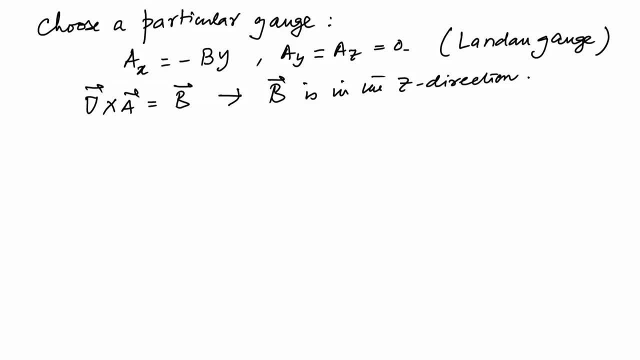 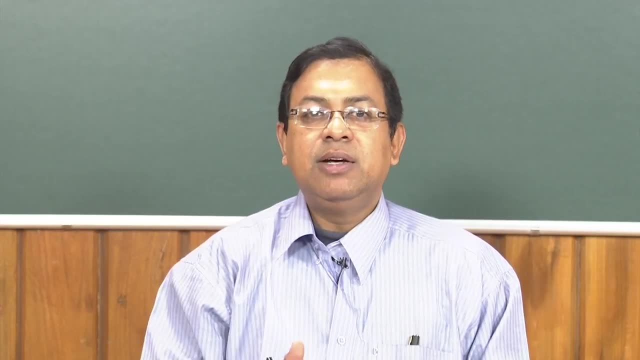 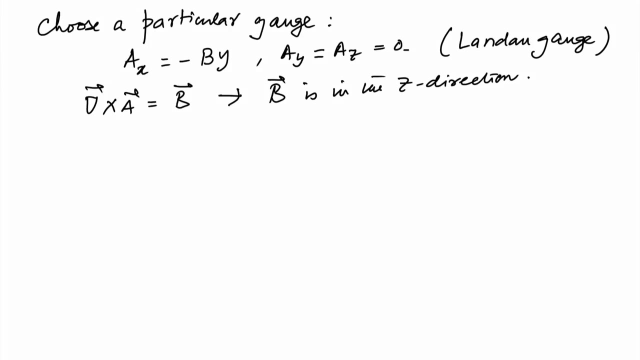 three dimensionality Schrodinger equation, but, however, very soon you will see that it boils down to actually a two dimensional motion and the B is actually pointing. the external magnetic field is pointing in the Z direction And if that is the case, then in this gauge Schrodinger equation I 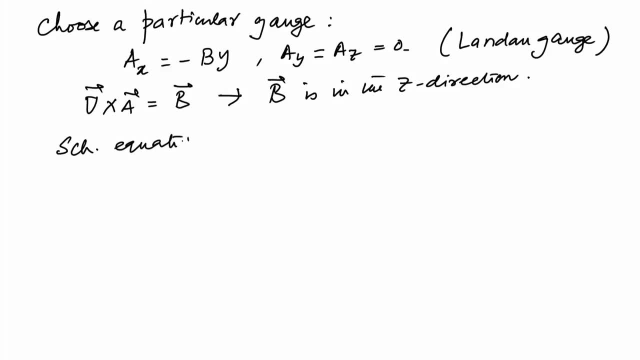 am writing it in short. So it becomes equal to 1 over 2 m, P x minus E, b y whole square plus P y square over 2 m, plus a P z square over 2 m and a psi of r, Which is equal to E psi of r. So, as any quantum mechanics problem we have to find 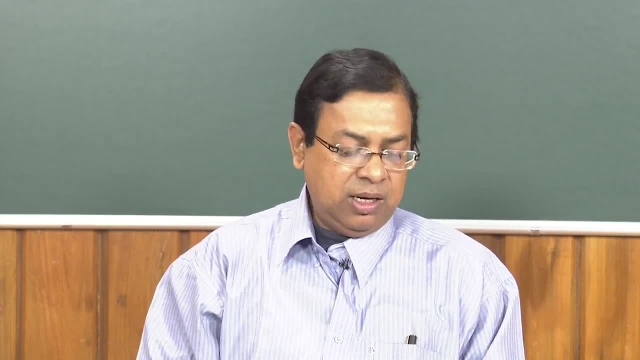 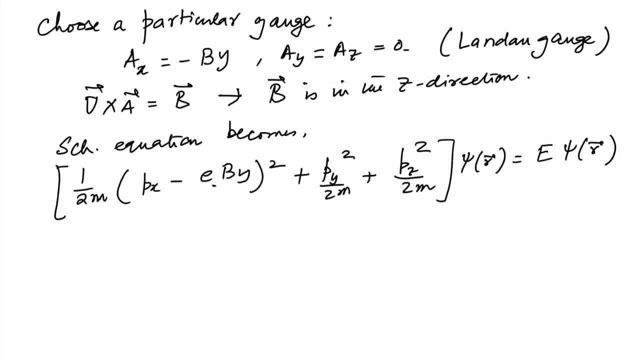 out the eigenvalues and the eigenvectors for this particular equation. So you can see that the Z direction, the particle motion, is like a free particle. So we have the energy in the Z direction is like a free particle And there is no other term which involves Z. So the motion is that of a free particle. 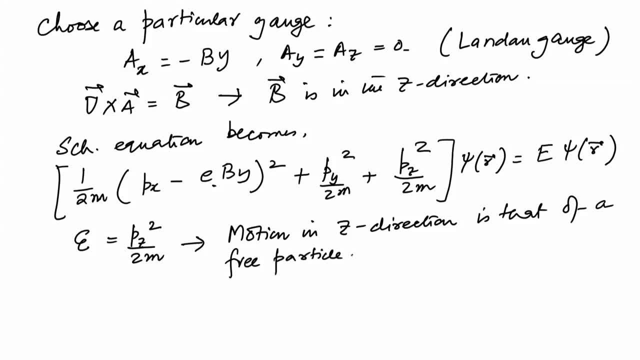 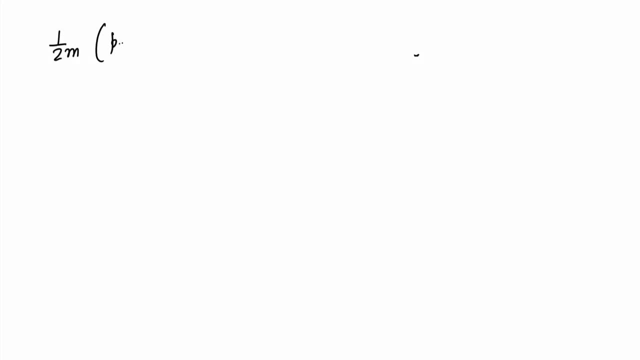 So now we can now neglect the Z direction, because it is like a free particle, and see what happens in the x and y direction. And to see that let us write down: p x minus E, b y square plus P y square over 2 m. And now the wave function. let us call it as f x, y. 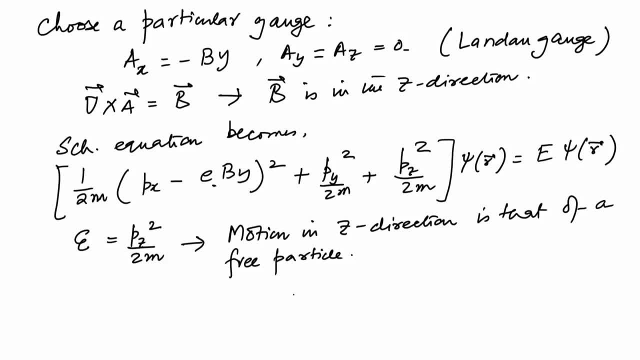 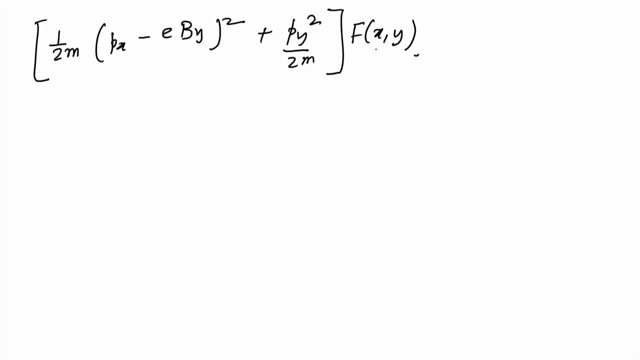 is no longer a function of z, because in the z direction the wave function is like, let us call it as say: f of z is some, with some normalization. it is like exponential i k, z. So we are only concerned about the 2 dimensional motion, and this is what we were talking about earlier. 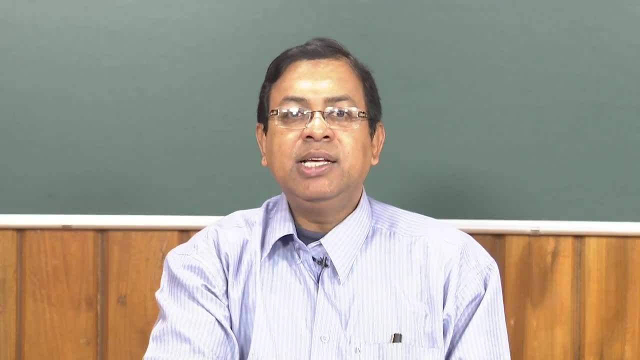 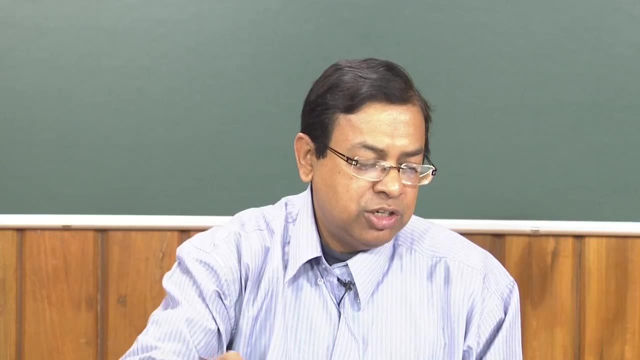 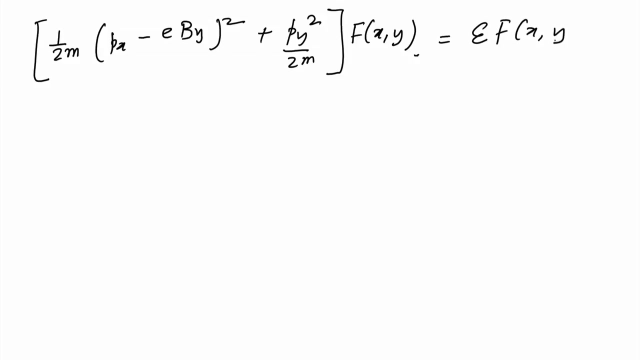 that even if you have taken 3 dimensional case in presence of a magnetic field for a non interacting electrons, it boils down to a problem of 2 dimensional motion and this is equal to some epsilon and f, x, y. So this is like the Hamiltonian in 2 dimension. 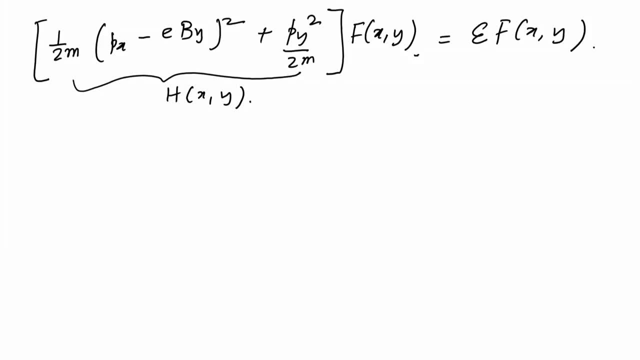 H, x, y. it is easy to see that P x is a constant of motion. Why P x is a constant of motion? because nowhere in this Hamiltonian we have x, The variable position, variable x, and P x is equal to this is equal to 0. So that tells: 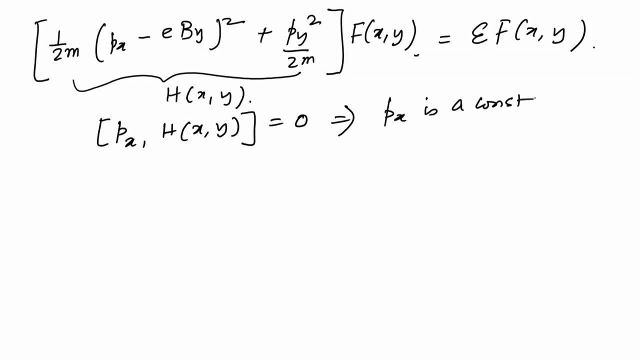 that P x is a constant of motion. Remember: P y is not a constant of motion because of the gauge chosen, where we have a y remaining. So P y does not commute with y and hence it is not a constant of motion. So there is no term, because there is no. 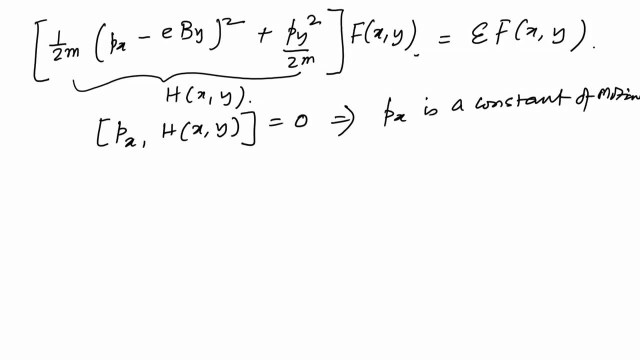 term linear in x. this is what happens, and that also, as I told, because of the gauge, but it does not matter. even if you would have taken a term a to be B x, then the x would have been P, x would not have been constant of motion, while P y would have been So x. 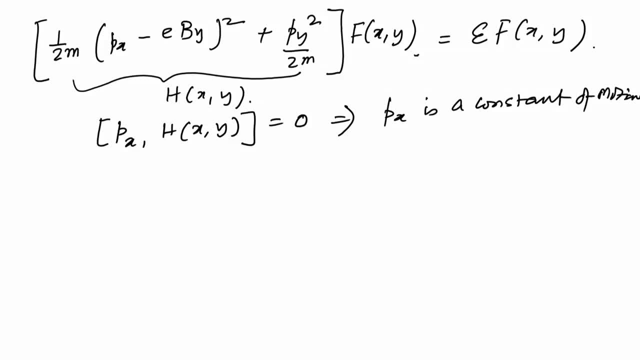 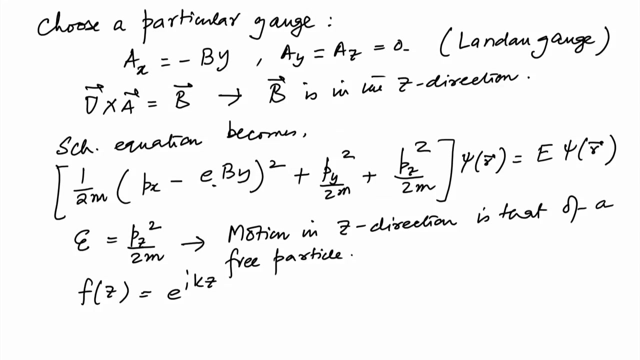 and y simply gets interchanged. So if P x is a constant of motion, then P x is actually quantized by this form, where n x is, of this, quantized in this form, which is, which takes values which are like 1,, 2,, 3 and so on. So one can write this equation. let us call this the original equation. 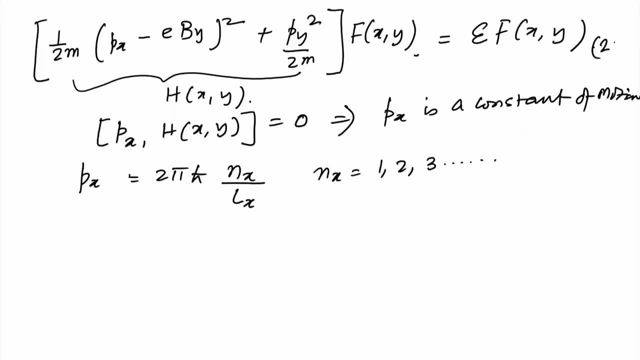 to be 1 and this equation to be 2.. So one can write equation 2 as p y square over 2 m plus half m, E b over m square y minus y, 0, square f of y, which is epsilon f of y. So 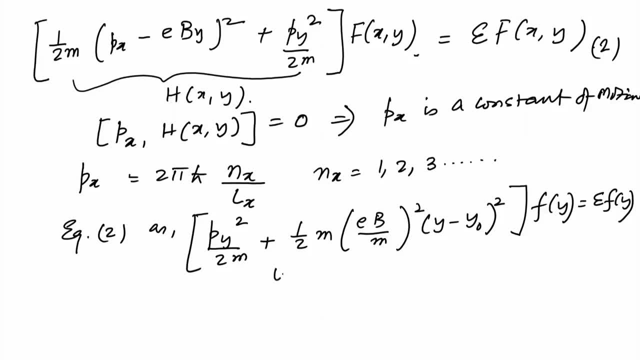 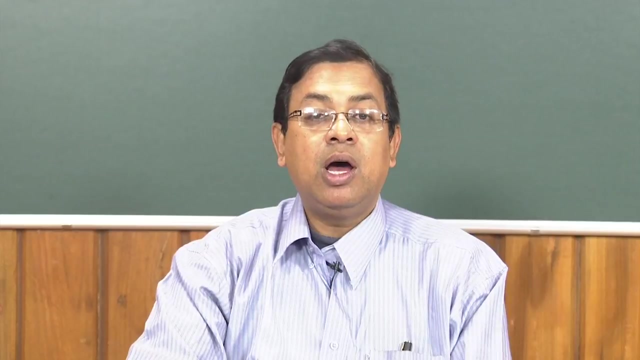 this is the equation Where y 0 is equal to p x over E b. So that is the equation, that is the Schrodinger equation that we have to solve, and it is very clear that this equation is the equation for the same equation. same Schrodinger equation when written for harmonic oscillator in the y direction. 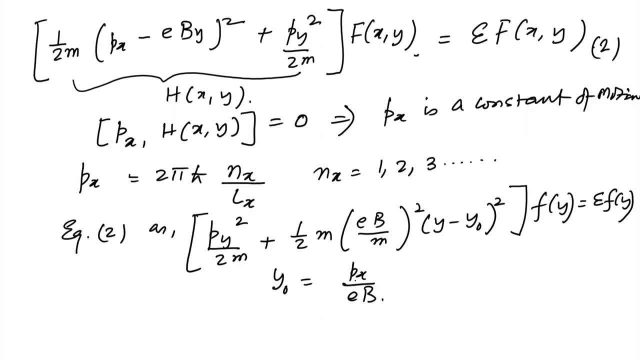 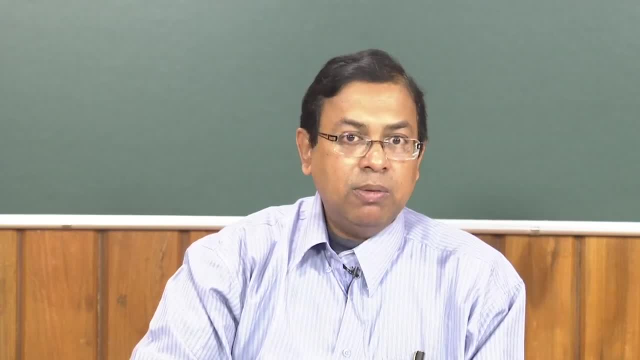 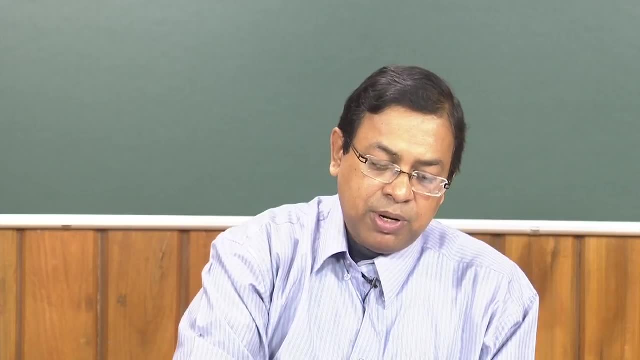 and oscillating about this point: E 0 given by p x. So this is the equation by E, b, and then, of course, we know that we have solved the problem in the sense that we know that it is of the harmonic oscillator form. So it is simple. 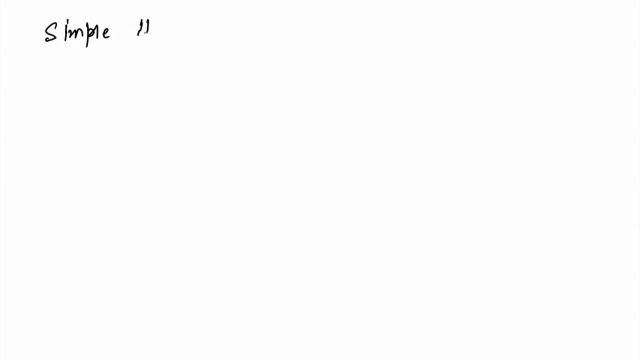 harmonic oscillator frequency E b over m. So the Eigen values are simple: epsilon equal to n plus half E b by m and h cross. So that is our. So it is n plus half h cross, omega and omega is given by this. So this is the Eigen value for this problem. 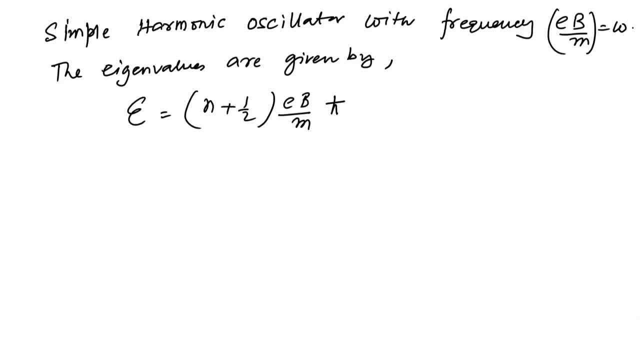 and these are called as the Landau levels. Not only we know about the energy Eigen values, we also know about the Eigen functions, So the two-dimensional Eigen functions. So it is a free particle. we told that the k, x, h commutes with p, x or 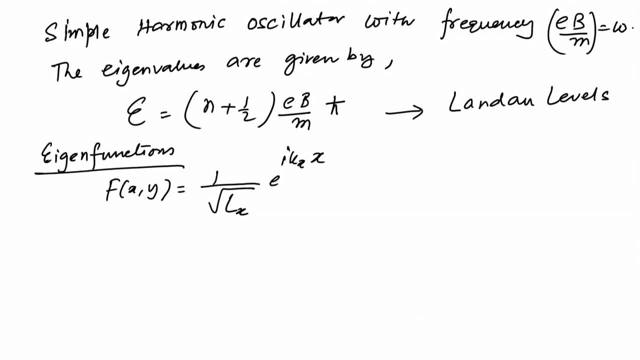 k x. So it is a free particle in that direction, in the k x direction, and some normalization. this is the Gaussian which is E b by y minus y, 0 square divided by h cross. and now the Hermite polynomial must be: knowing the properties of the Hermite polynomial when n equal to 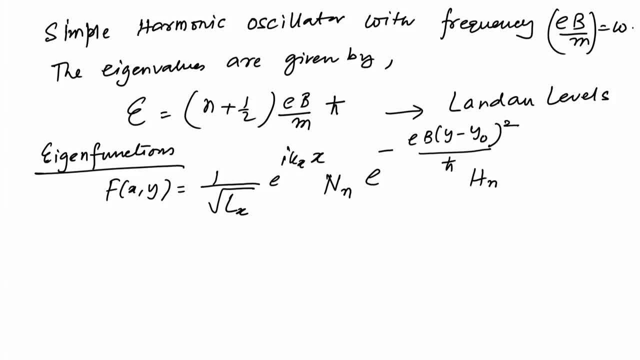 even the polynomial is, even when n equal to odd, the polynomial is odd and it is given by y minus y 0 divided by h cross, and that is the complete solution of the problem. There are more things to understand here. is that So these are Landau levels and these 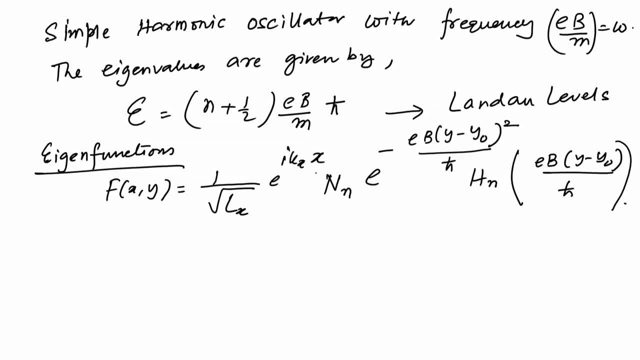 are the Landau level energies. and now you see that a p x is a constant of motion. So that tells that all n x that satisfy all n x that satisfy this quantization condition, 2, pi n x over L x, Where y 0 equal to h, cross h, sorry, h over B L x into n x, all n x values are valid solutions. 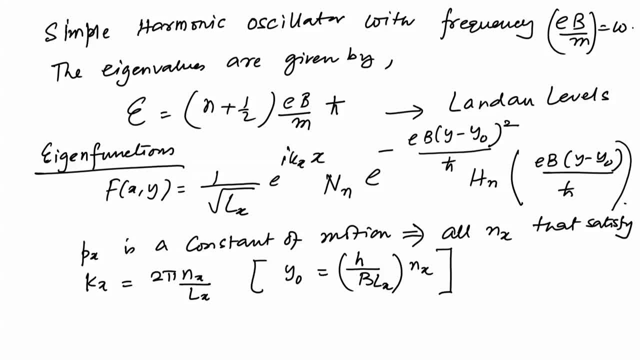 and since all n x values are valid solutions, the problem is hugely degenerate and gives rise to the enormous degeneracy of the Landau levels. Because each N x value that satisfy this relation- L x is the dimension of the sample in the x direction- will be a valid solution, and hence 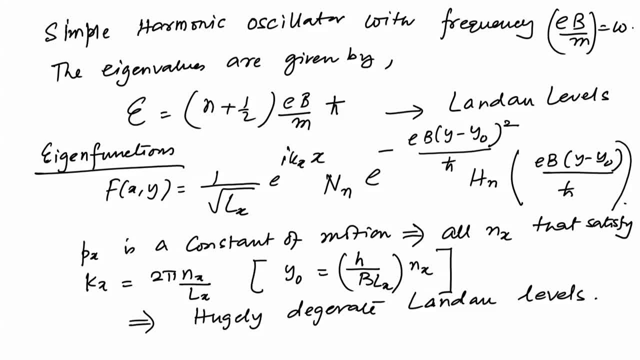 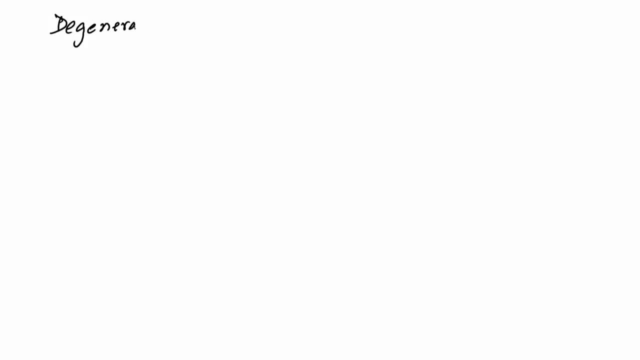 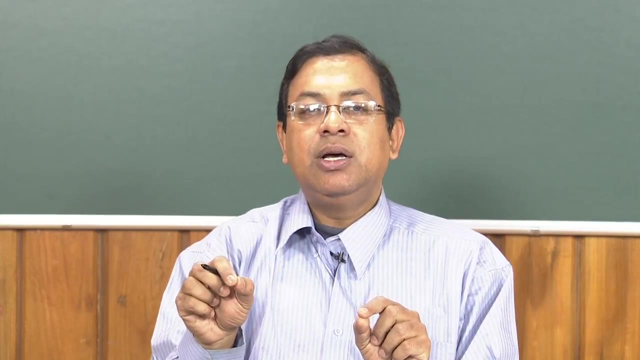 it is a enormous. this degeneracy will be there. Now, what is the extent of degeneracy? So let us try to understand. So let us take this energy value. So your y is y naught. So this is the point about which the particle is undergoing simple, harmonic motion. So 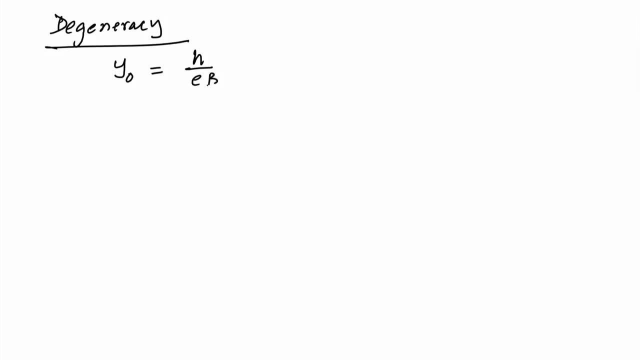 this is given by h over E b into k x and of course, as I told that k x is written as 2 pi, N x by L x. So my N x max is given by k x max and divided by I mean k x max. 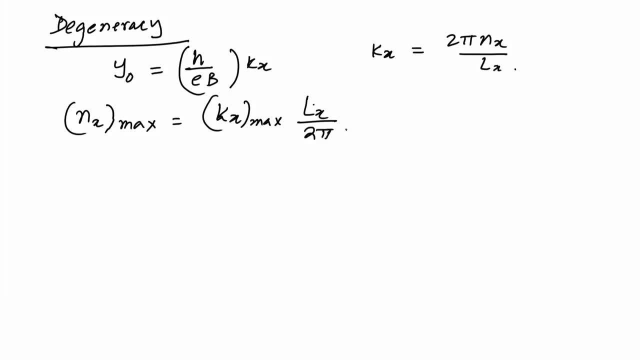 into L x by 2 pi. Now, if we put that, this k x max here, and take y 0, which is the point in the y direction, So this is the point about which the particle is undergoing simple y direction, about which the simple harmonic motion takes place to be the. So take y 0. 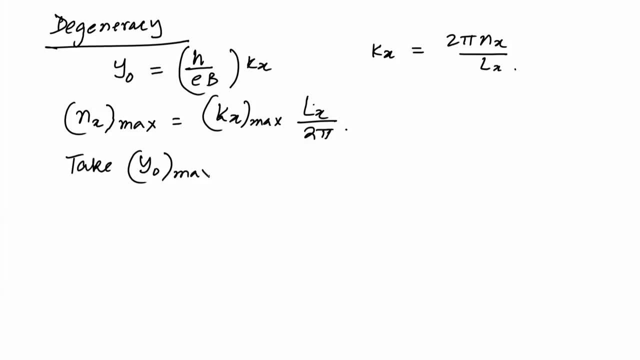 max equal to L y, which is the size of the sample in the y dimension, y direction. So it cannot- y 0 cannot be greater than L y. So the particle is undergoing a simple harmonic motion about y 0 and y 0. the maximum of y 0 is the sample dimension in the y direction. 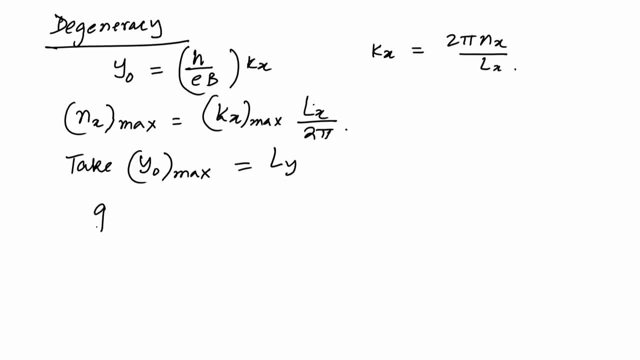 So the degeneracy is then given by: g is equal to N, x max, which is equal to E b, L, x, L, y divided by h, which is equal to E b, by h, into a, where a is the area of the sample. 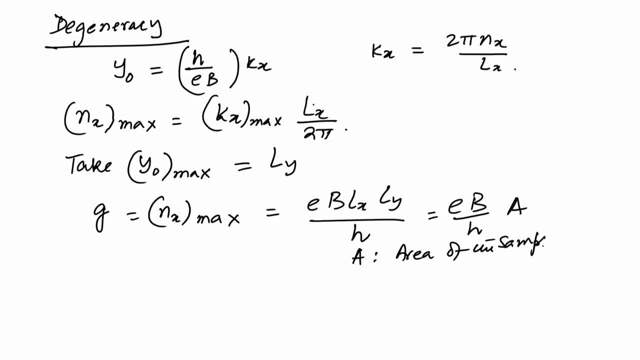 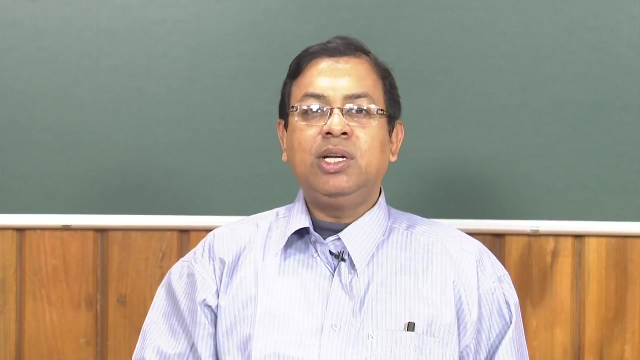 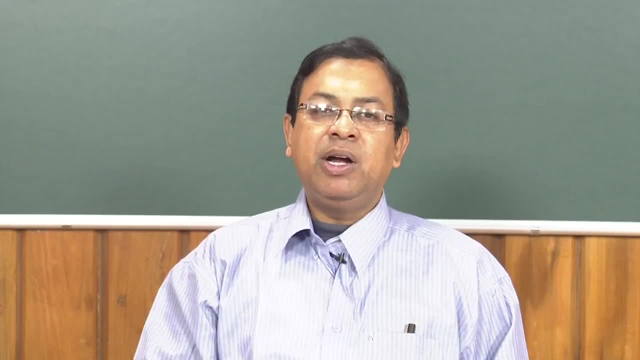 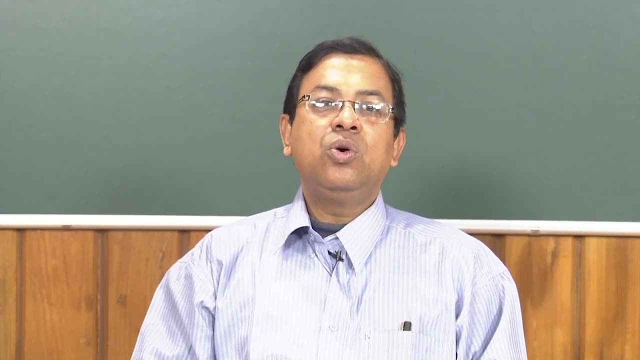 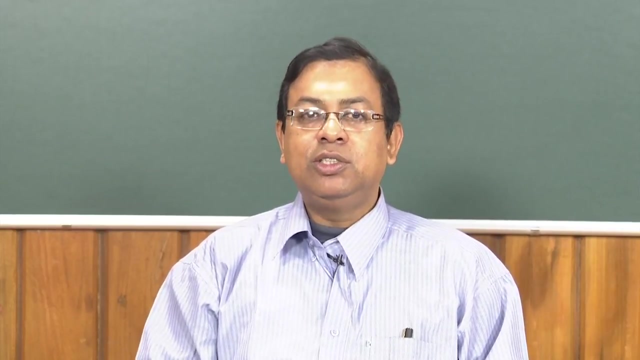 The problem says that the motion in the z direction is that of a free particle, So one can neglect that. So now the Hamiltonian becomes two dimensional, and so the motion is constrained in a plane in the x direction because of the choice of the gauge, the particle. 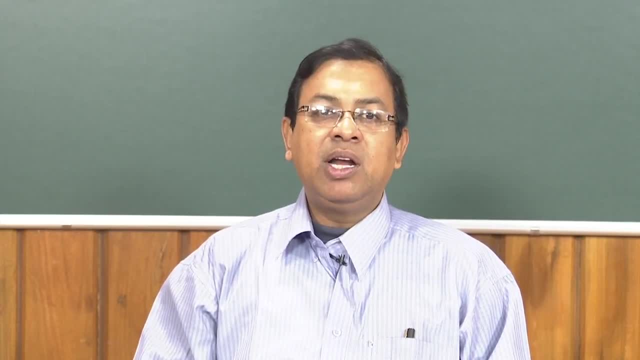 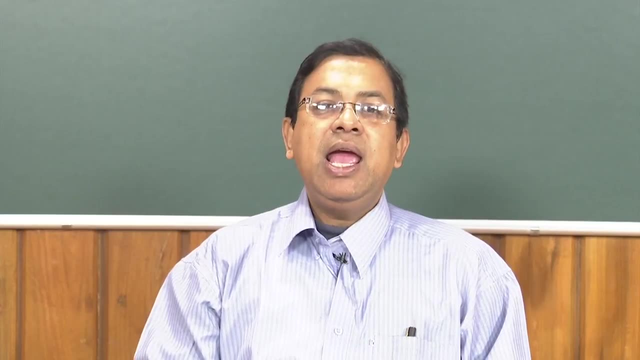 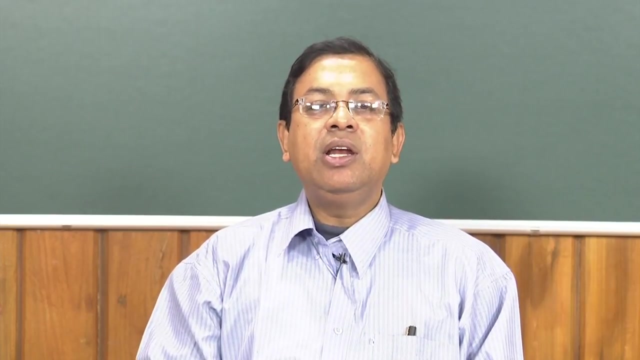 moves as free particle with the momentum vector quantized in terms of 2 pi over L, some integer multiple of 2 pi over L, and in the y direction it executes a simple harmonic motion. So we can find, we can we get this effective Schrodinger equation is a one dimensional Schrodinger. 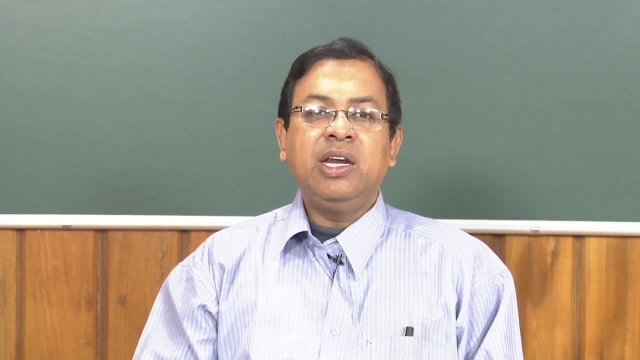 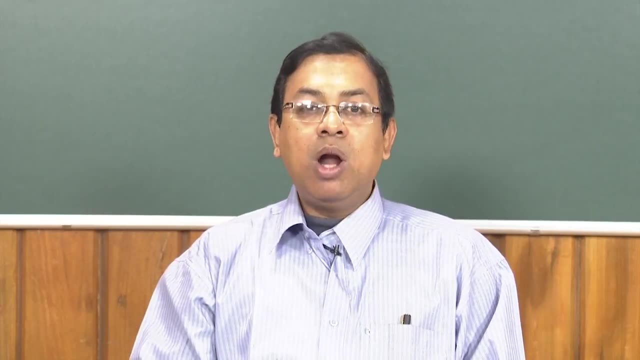 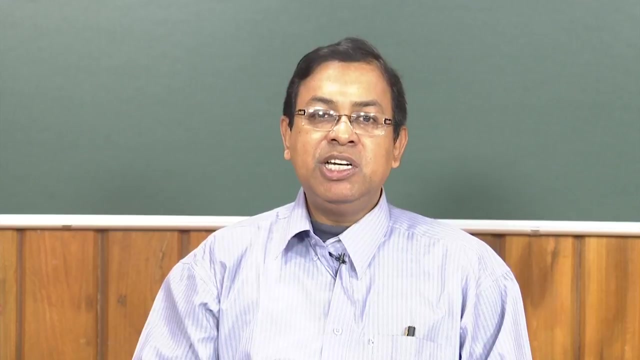 a simple harmonic oscillator problem. We know what the energy Eigen values are. we know what the energy Eigen vectors are, because any quantum number in the x direction is provides a valid solution for the problem. The problem is enormously degenerate and these degeneracy is found, and this degeneracy is proportional to b and it is also proportional to the area. 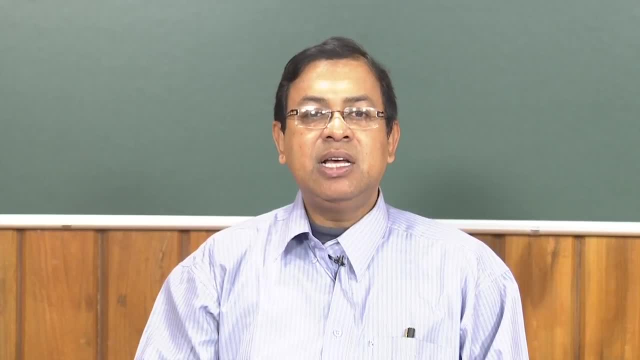 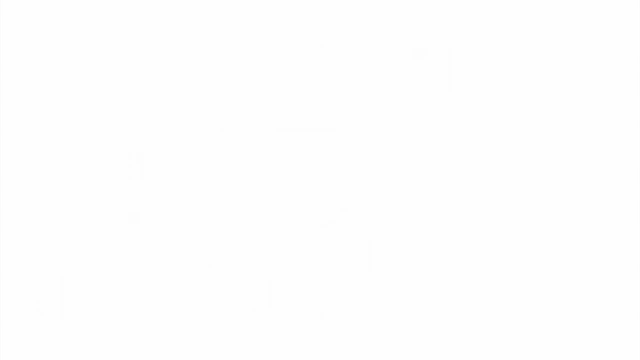 of the sample, and the trajectory is a simple harmonic which is centered at y 0.. Now, with this, so having discussed this Landau levels and degeneracy, let us talk about how this problem. now you should be finding a similarity between this problem and the quantum Hall. 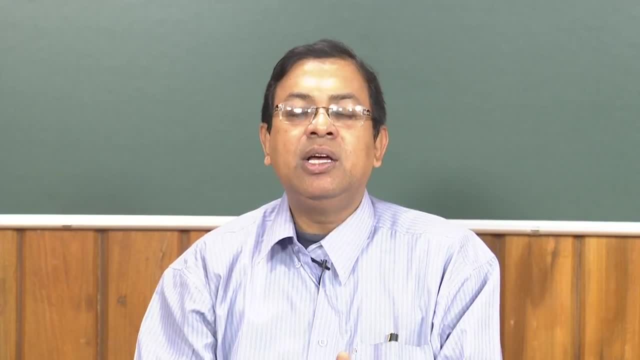 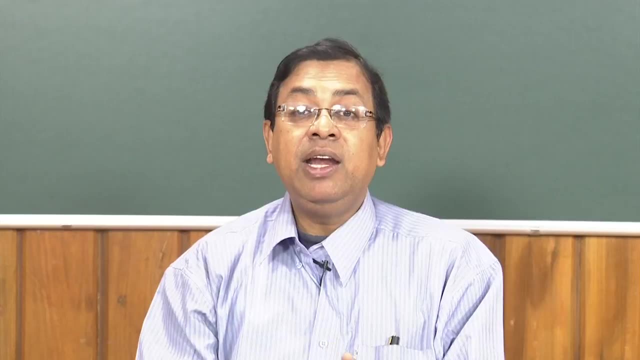 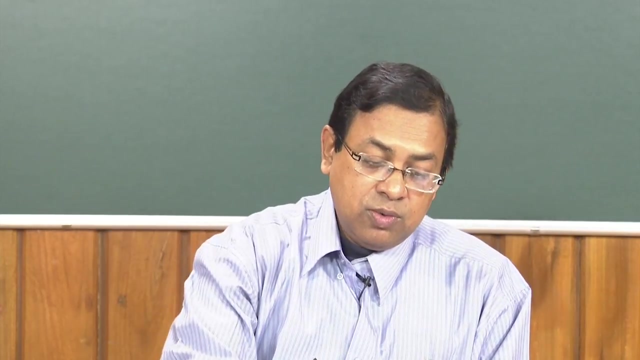 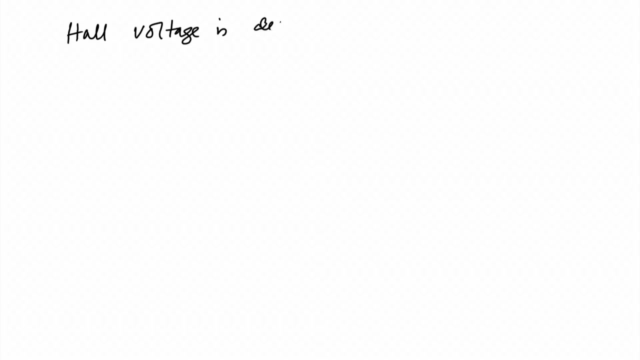 effect. There also, the electrons were put in a strong magnetic field in the z direction. here also we are talking about a single electron and finding that how the motion is in a presence of a magnetic field. So now the Hall voltage is different from. 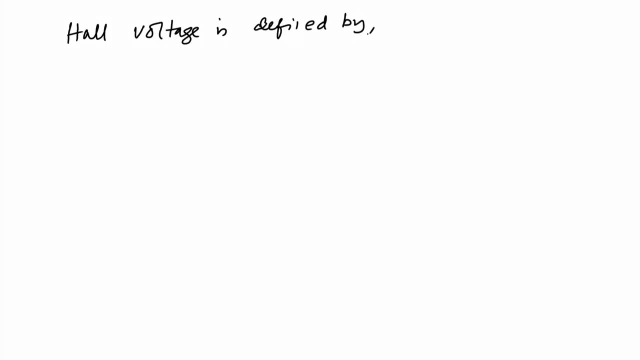 a magnetic field. So this is defined by v h, which is equal to b, i x, over n e, and hence the Hall coefficient R h, which is equal to v h, by i x, this is equal to b by n e. So this is a classical result which is well known. So the degeneracy of the Landau. 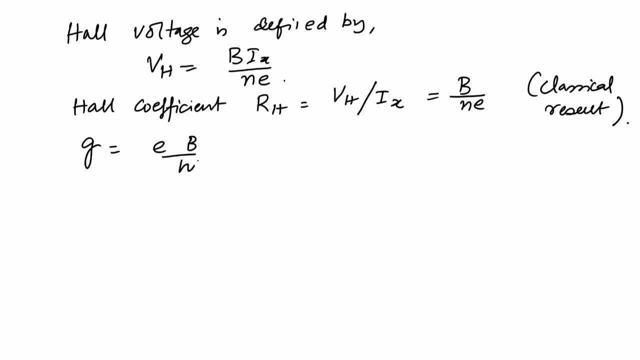 levels is given by e, b, by h into a. So the degeneracy. so this is the degeneracy. So degeneracy per unit area. So R h. let us do it in a new page. then R h becomes equal to n h divided by nu, n e square. 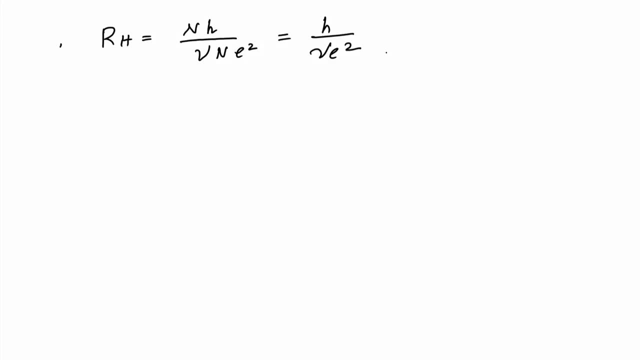 it becomes equal to h by nu e square. So nu becomes equal to n by e b over h. So this was the quantization that was discussed at the beginning of the Ah of the lecture. So, even starting with a classical picture, if you think that this, 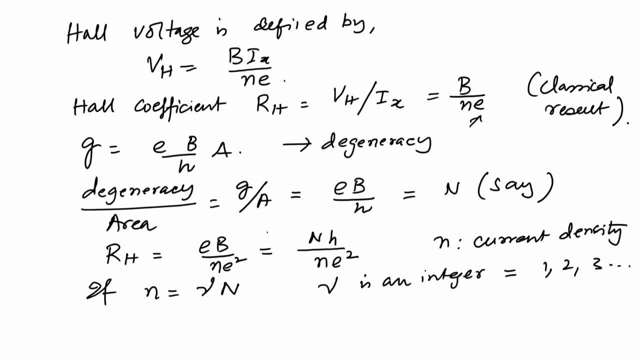 the assumption is that if the degeneracy per unit area is quantity, which is like, you can take it as a number, as n, and then the Hall resistivity, it is quantized in terms of h over e square, it is a, where n is the electron density, it is n h over n e square. and if a n is taken, 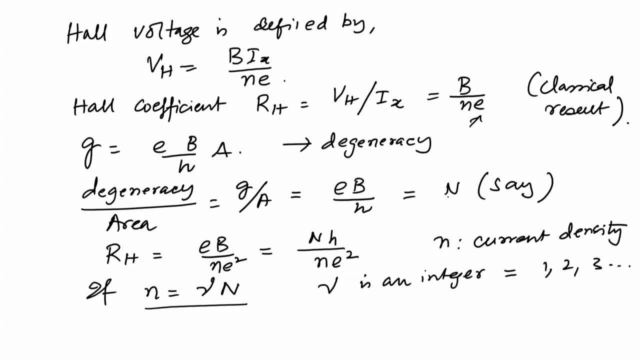 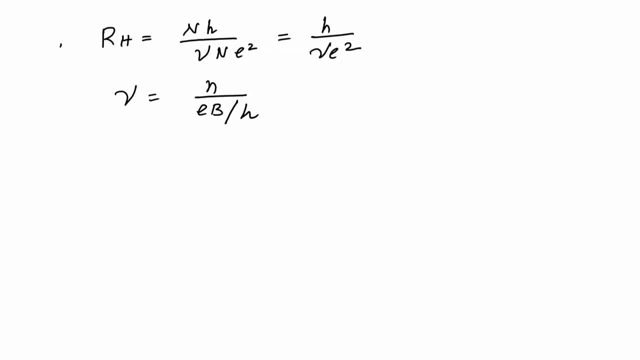 as the gamma into this capital N, which is taken as the degeneracy per unit area, then it is quantized actually as h by e square and 1 over nu. So thus a quantized Hall resistance is always expected. this is important. 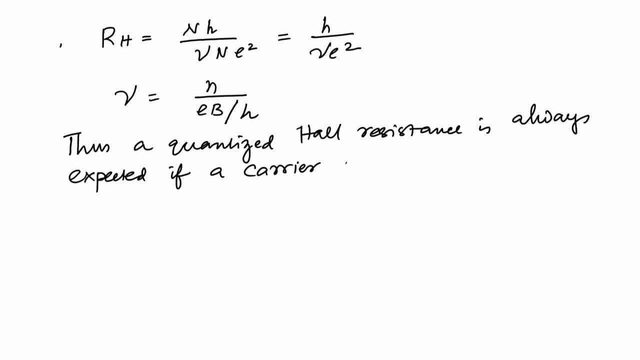 If a carrier density, If a carrier density n, n and the magnetic field B, B are adjusted in such a way that the filling factor- this called this, nu, is called as a filling factor. nu of the Landau levels satisfies nu equal to B welfare condition. hundred percent and seized carsemptly, And this is called Joulet. ratio between lambda and vu mean: multiply by Trying of 40 degree c into min plus one equal to zero. Is that clear Right Selectively? Did we all get this? we have a setup that in X I 데 respect the地方s this way. then C to 2. opportunity is that those essentially calm. a class in z belongs to an ting poder c minus A Beim does not. That does not to allow you specifically able to rely on the s, namely random. 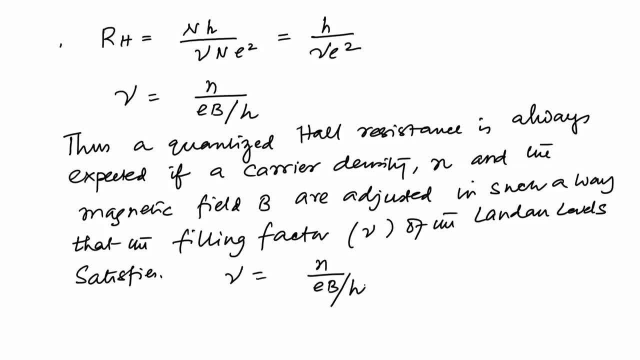 to N by E, b, H becomes an integer. So it is satisfying this becomes an integer. So just to rephrase this, that even from a classical picture we got this quantization of the plateaus or the Hall resistivity or the resistance. Here what we have taken is: 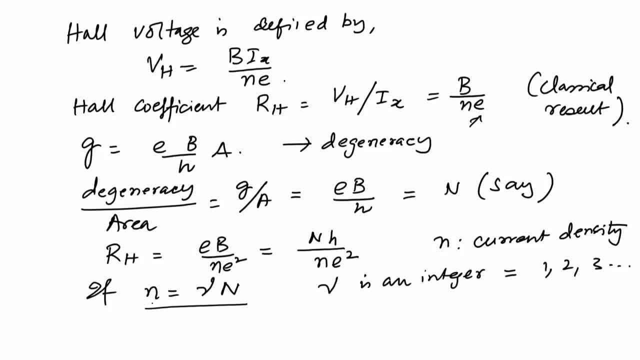 that this is called as a filling factor, where the total electron density is taken as filling factor, multiplied by the degeneracy per unit area. So your gamma is simply equal to N by N. So that is the electron density divided by this N, which is the degeneracy or the degeneracy. 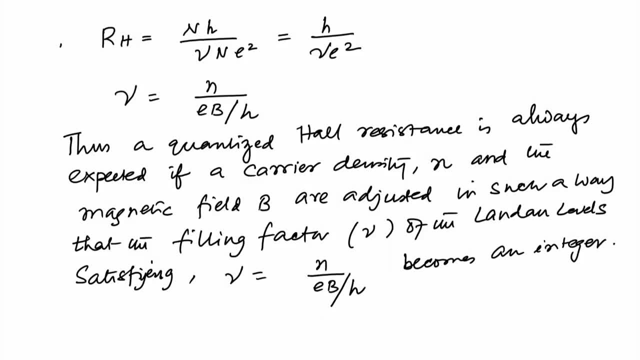 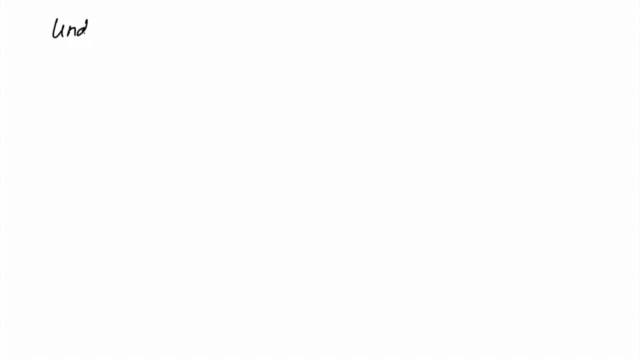 per unit area. If these two things and the b that can be adjusted in a manner such that this quantity becomes an integer, then there will be quantization of the Hall resistance. So what happens is that under this condition, the magneto conductivity, let us call it as 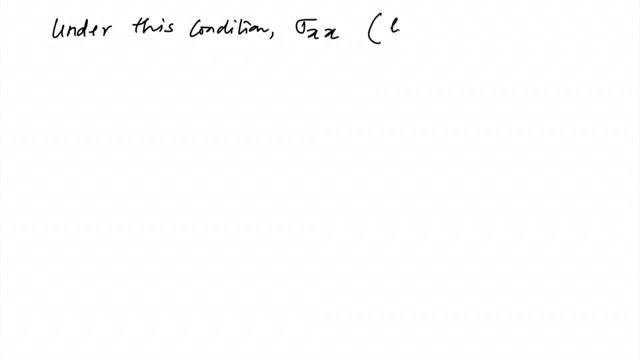 sigma xx. So we have got that the electrons in the x direction, that it moves like a free particles exclusively perpendicular to the, to the electric field. Thus there is no scattering in the direction. in the direction of the electric field is possible. So whenever rho xy acquires 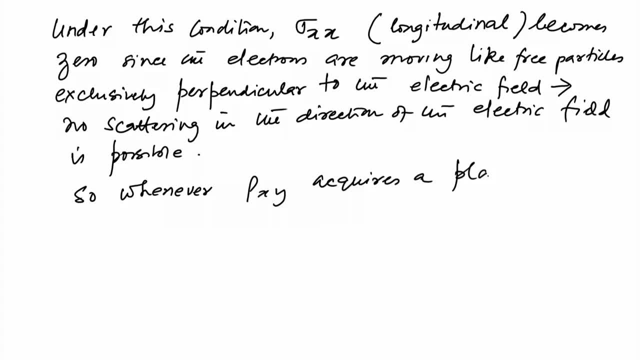 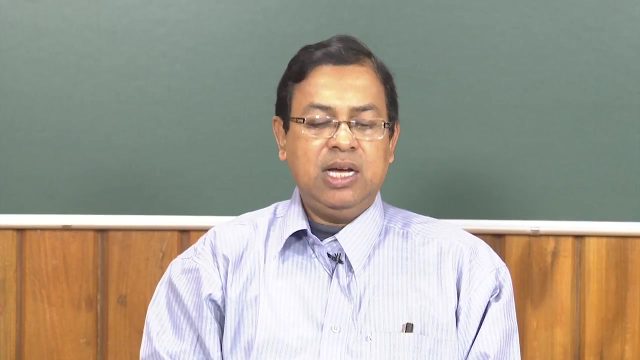 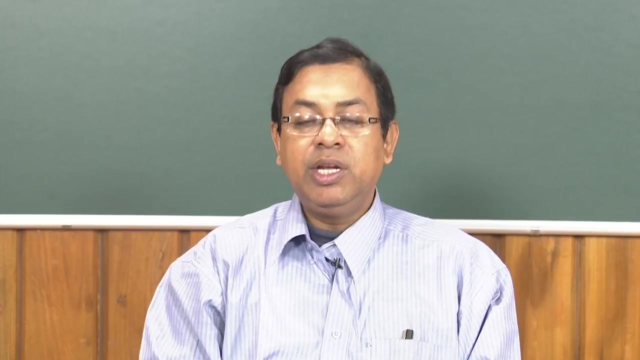 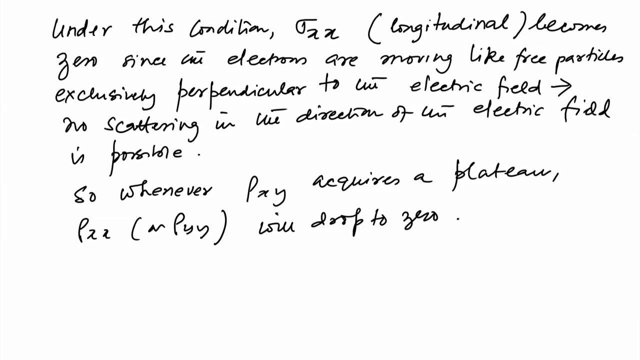 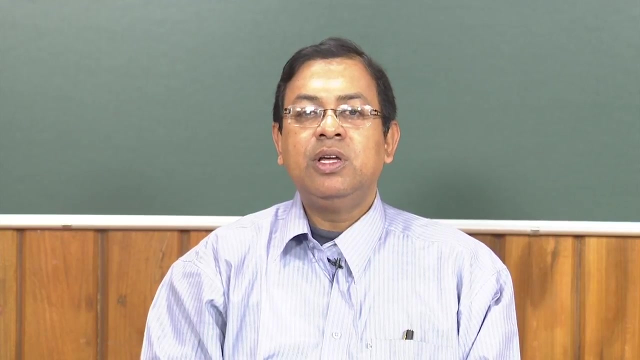 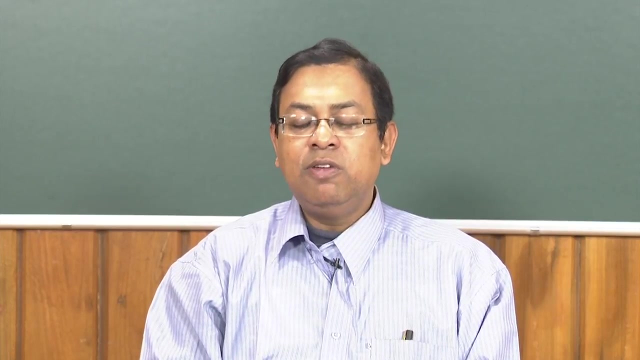 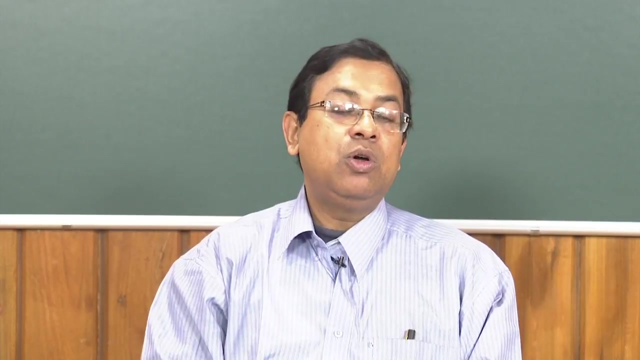 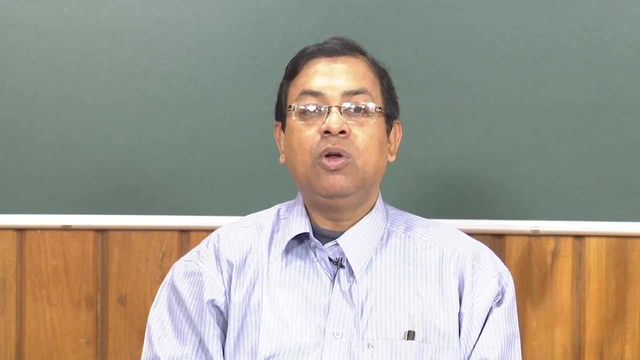 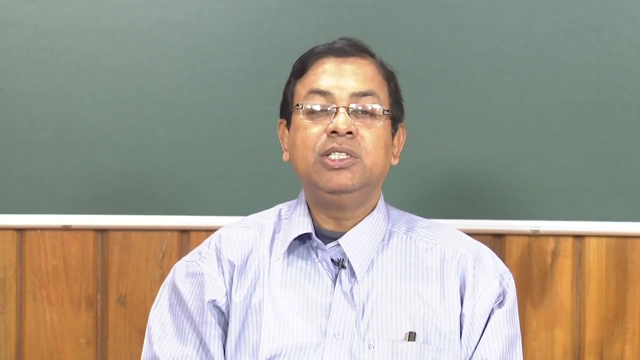 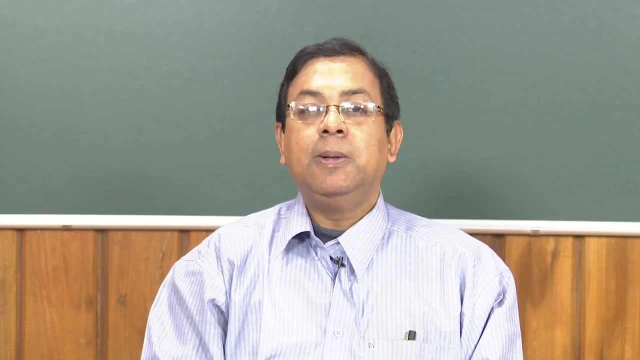 a plateau of resistivity is there. people do the Hall effect measurement almost on any sample that comes, because it gives rise to not only the magneto resistance or the magneto conductance, also the Hall resistance, and helps us in understanding the quantization of the plateaus.